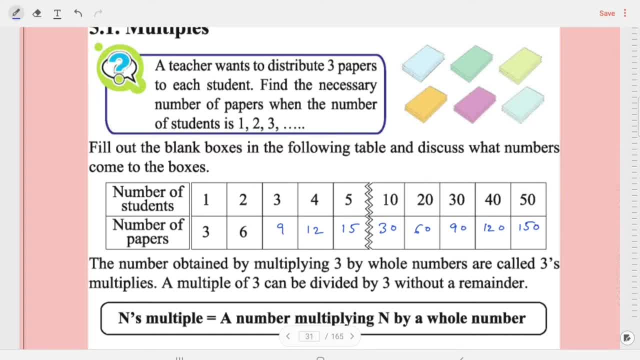 For example, 6, 9,, 12, 15.. You can divide all these numbers by 3 without any remainder. So what is n's multiple, then? A number multiplying n by a whole number. That is the definition of multiple. 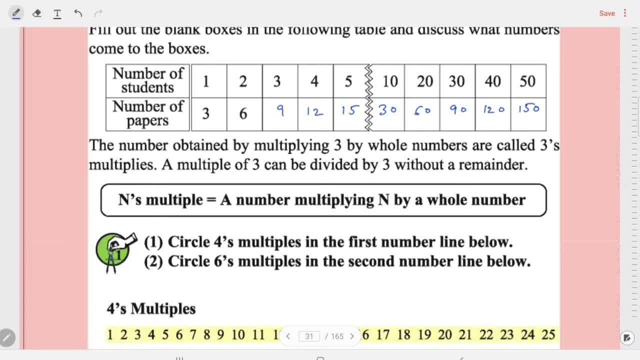 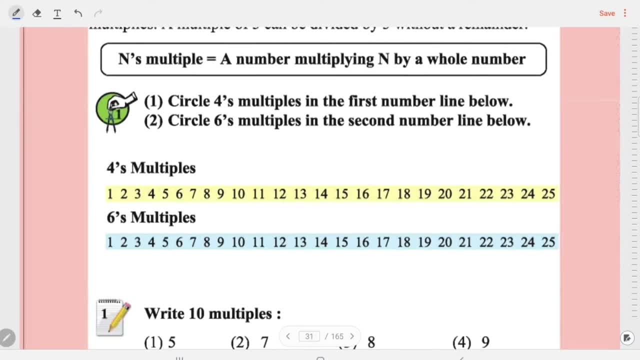 Circle 4's multiples in the first number line below Circle 6's multiples in the second number line below Circle 4's multiples first: 4, 2x8,, 4,, 3x12,, 4,, 4x16,, 4,, 5x20,, 4,, 4,, 4x6,, 4x24.. 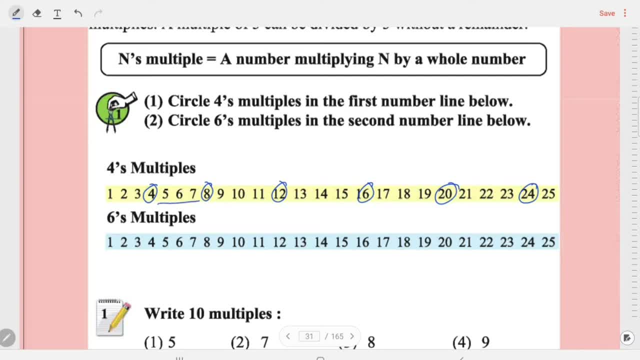 If you carefully observe, the distance from here to here is same: 4 plus 4.. 3 numbers come in between. Likewise, here also, The distance is going to be same. What about 6's multiples? First is 6,, then 6,, 2x12,, 6,, 3x18,, 6,, 4x24, and so on. 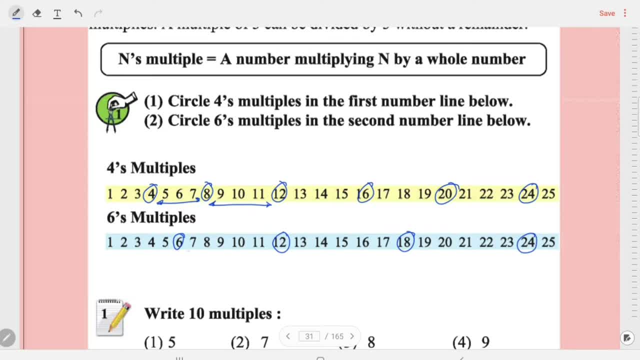 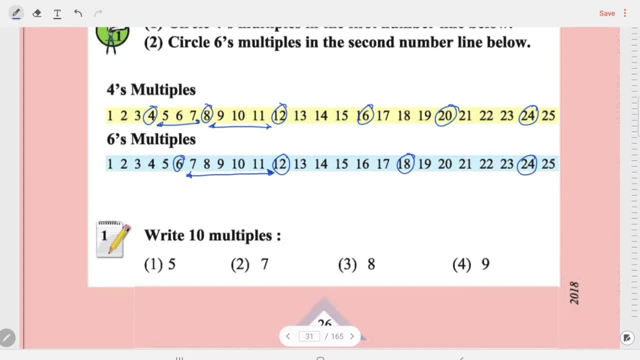 Here also, you can see, you can count the distance: 6 plus 6 is 12.. So in between there are 5 numbers. Okay, Alright, Alright. 10 multiples: 5x10 is 50,, 7x10 is 70,, 8x10 is 80,, 9x10 is 90.. 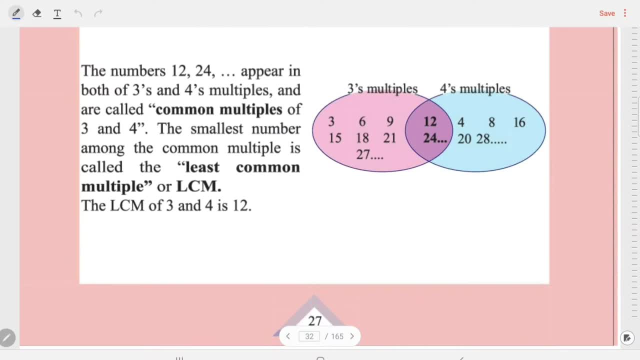 Alright, The numbers 12, 24 appear in both 3's and 4's multiples, Okay, And are called common multiples, For example. For example, the numbers 12 and 24 appear in both the multiples 3 as well as 4.. 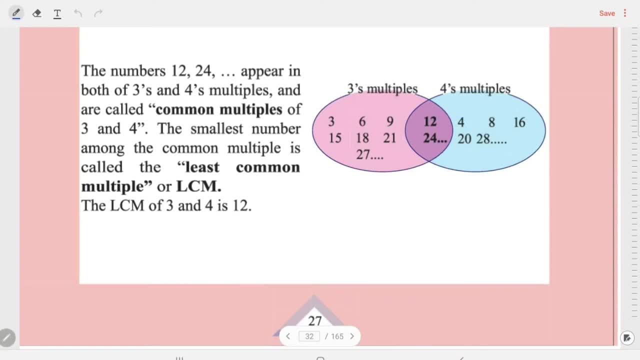 So these are the common. Okay, 3x4 is 12,, 3x8 is 24,, 4x6 is 24.. Like that, The smallest number among the common multiple is called the least common multiple. That is called LCM. 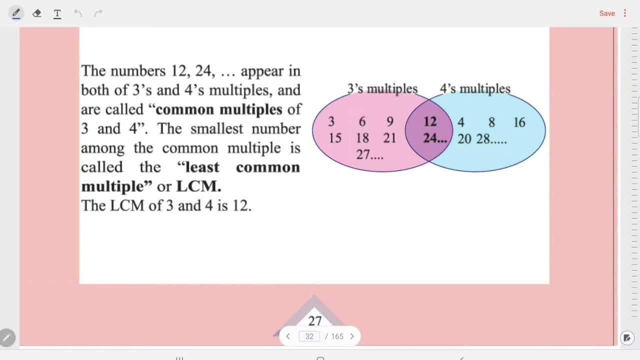 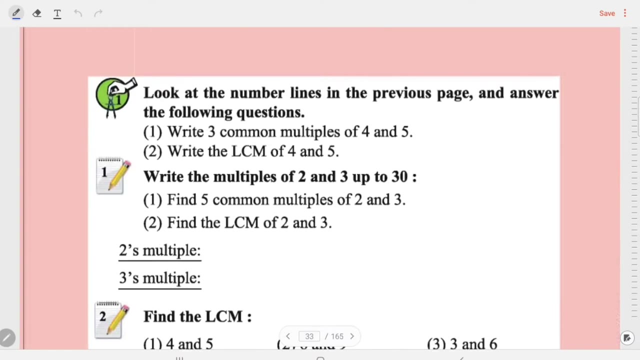 Okay, So the least common multiple of these numbers- 3 and 4, which are co-primed to each other- is a product of those 2 numbers, ie 12.. Okay, Got the point Right, Mhm. 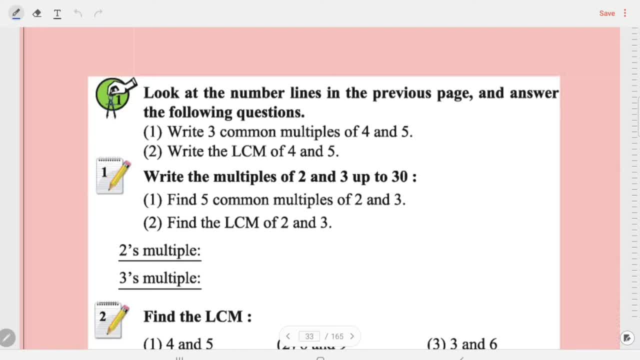 Look at the number lines in the previous page and answer the following questions. Right 3, common multiples of 4 and 5.. 4 x 5 is 21.. Okay, 40 also, you can. you can say 60 also. okay, write the LCM of 4 and 5. see these two. 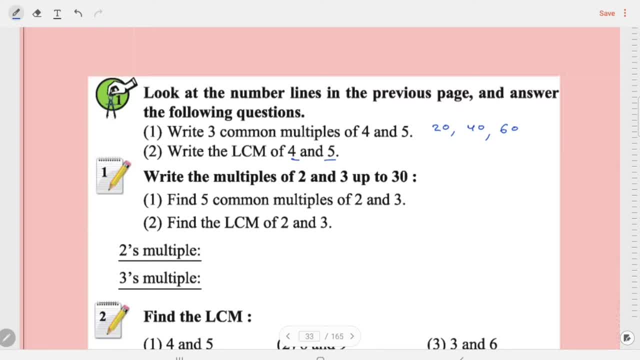 are co-prime. again, there is no count multiple among 4 and 5, so the LCM is just a product of these two numbers. when they are co-prime, okay, LCM of co-prime numbers is the product of the numbers. write the multiples of 2. 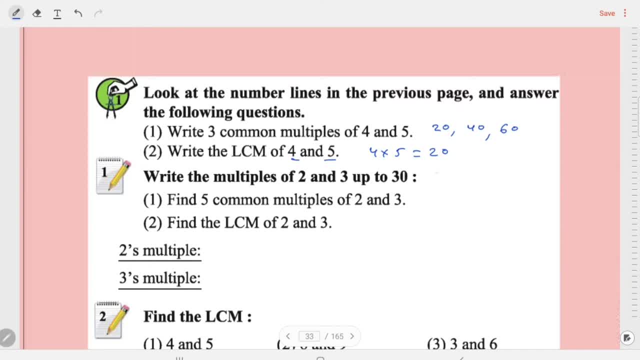 and 3 up to 30 multiples of 2 and 3. okay. 2, 4, 6, 8, 10, 12, 24, 26, 28, 30 here. 3, 6, 9, 12, 15, 36, 18, 21,, 24,, 27,, 30, ok, 27,, ok, ok, here. we missed some of the numbers. 14 is there, 16 is there. 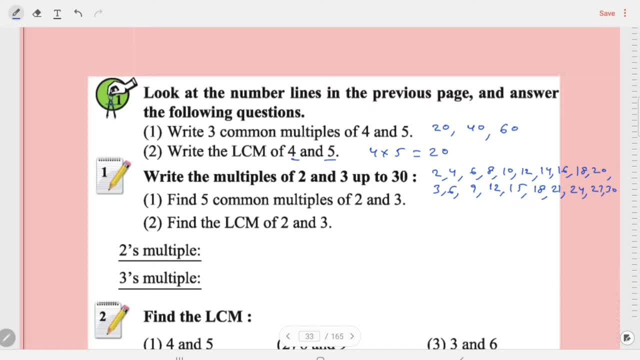 then 18 is there, then 20 is there. after 20- I am writing it here- 22,, 24,, 26,, 28,, 30,. ok, find 5 common multiples of 2 and 3, common multiples of 2 and 3, 6 is 1,. ok, we will. 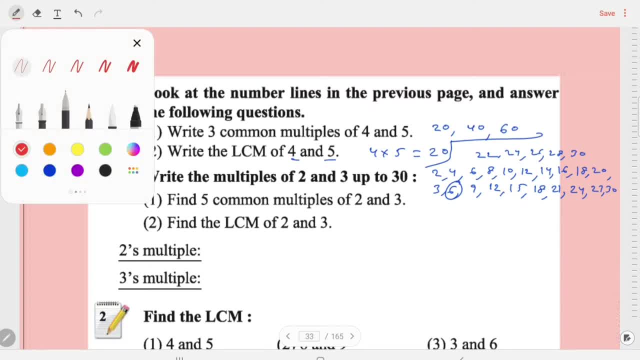 change the colour if you don't like to use the same colour. Ok, green is fine. 12 is there ok, and 18 is there ok. then 24 is there. 24 is there ok. 1,, 2,, 3,, 4,, 5 is there. 30 is there ok, fair enough. 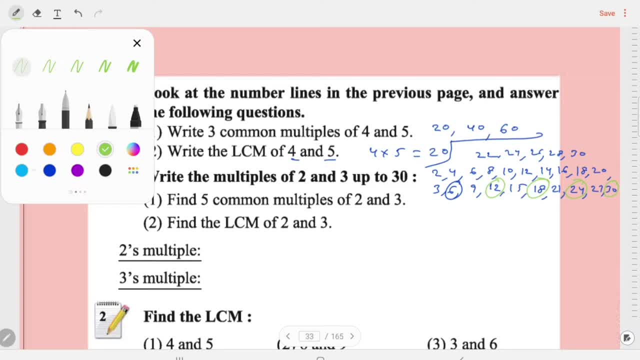 Ok, Find the LCM of 2 and 3, again change the colour to original colour: 2 and 3, these two are co-prime, so the LCM is 2 into 3, that is 6,. ok, want me to write it clearly. 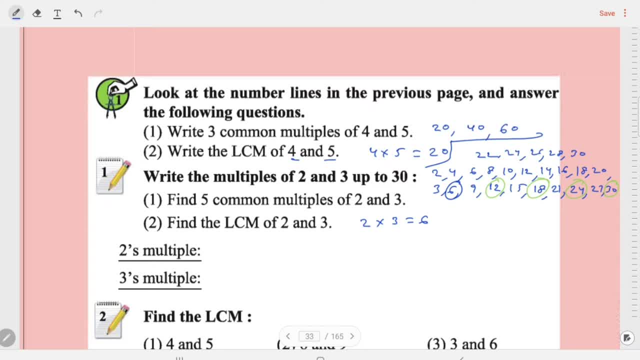 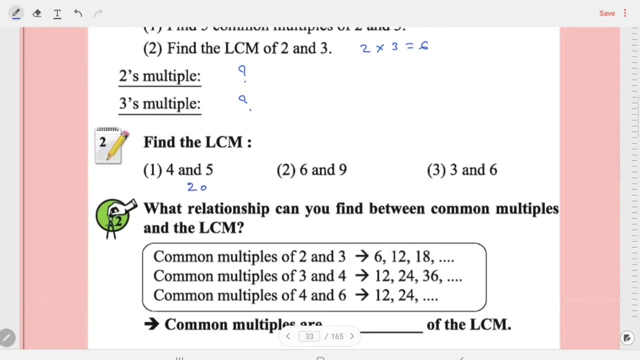 alright, 2's multiples and 3's multiples. ok, the space is given here to write these multiples, so write those multiples there itself. ok, Ok, 1 and 5,, that is 20,. what about 6 and 9,? LCM means least common multiple, right? the? 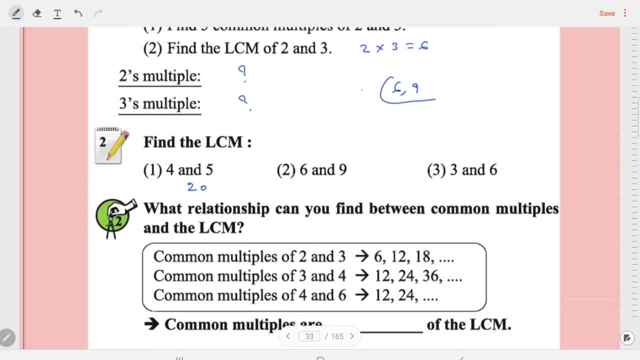 way to find LCM is like this: 6 and 9,. 2 is not a factor of 9,- ok, but 3 is a factor of both. so start with 3, 3, 2 is a 6,. 3, 3 is a 9,- ok, there are no common multiples here. 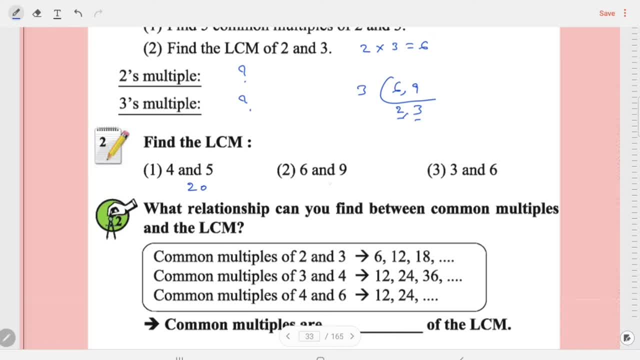 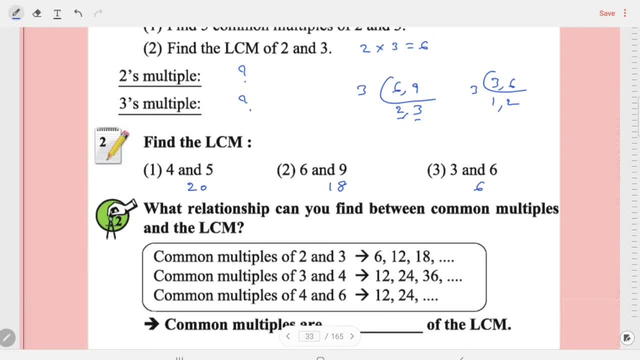 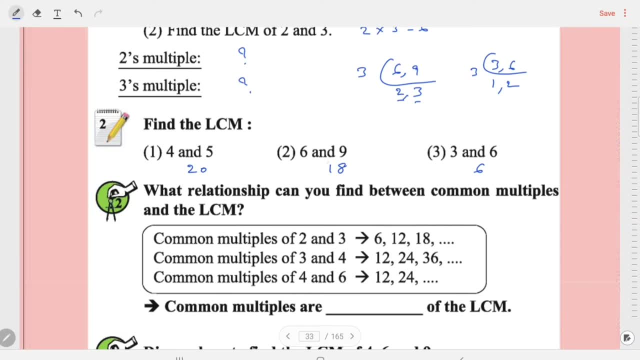 is a 6,. 6, 6 is the common, least common multiple. ok, like that you have to. you can check the answer as well. whatever the result you obtained must be the multiple of both the numbers. 18 is a multiple of 6, 6,. 3 is a 18,. 9 is a multiple of 18, because 9, 2 is a 18, so 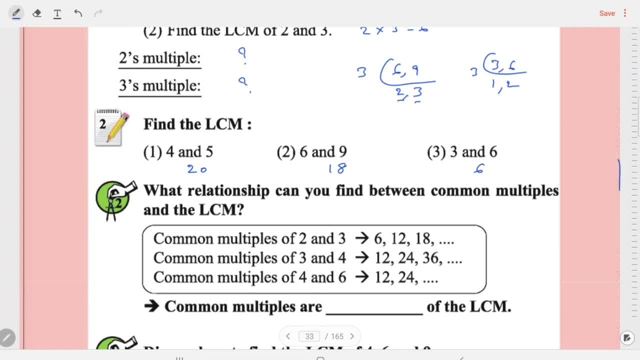 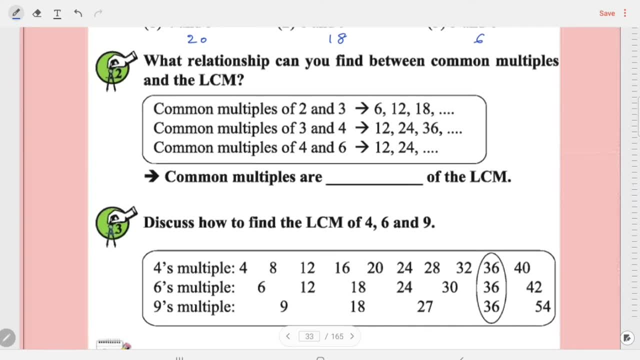 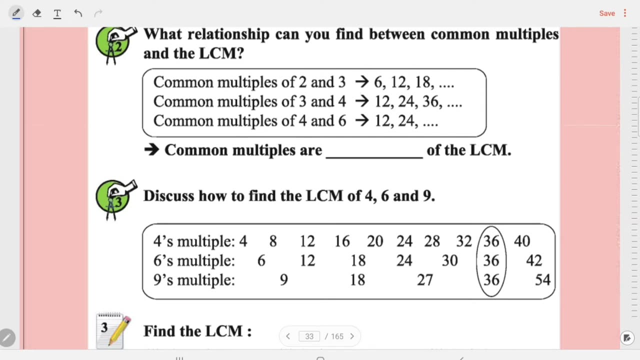 9,. 2 is a 18,. ok, likewise you have to check the answer also, right. what relationship can you find between common multiples and LCM? common multiples of 2 and 3 is this right? but what is LCM least common multiple? that is the first one and here also that should. 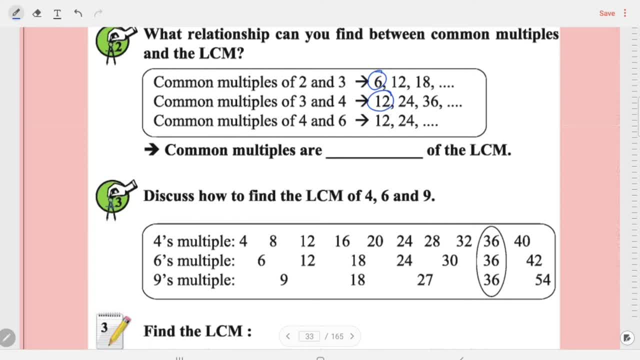 be the first one here also. Here also It is the First one, ok. so common multiples are dash of the LCM. so, ok, products of the LCM that we can fill right. see here: 6,, 2 is a 6,, 2 is a 12,, 6,, 3 is a 18,, 12,, 2 is a 24,, 12,. 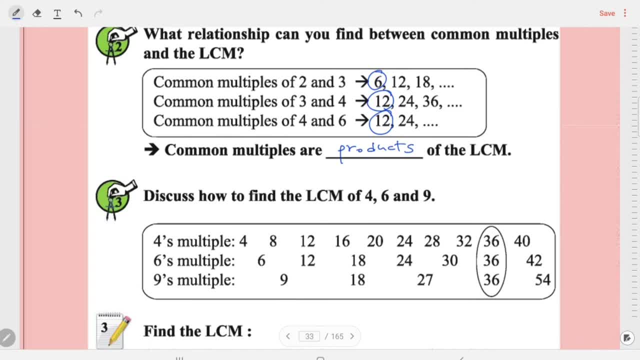 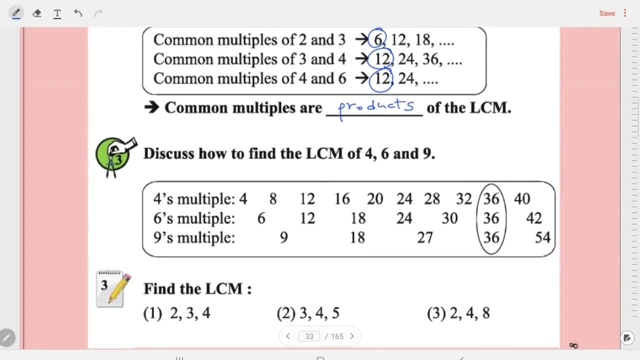 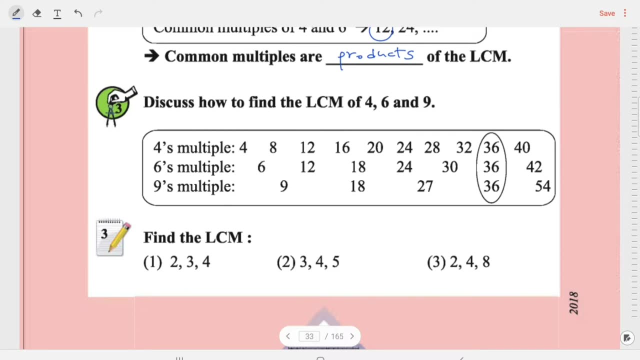 3 is a 36, like that. they are the products of the LCM itself. discuss how to find the LCM of 4,, 6 and 9,. ok, Finding LCM. I told you one method, but how the method arrived, how we came to such a. 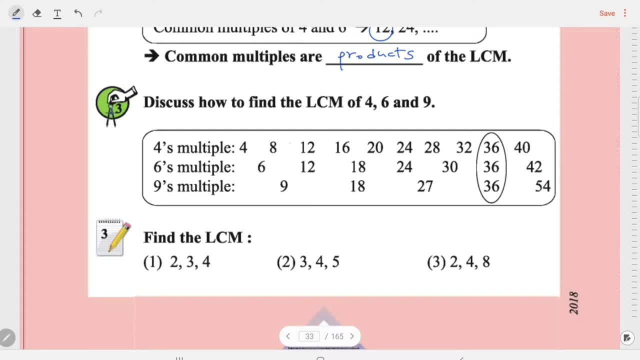 method. initially you should go like this: right: 4's multiple means 4,, 8,, 12, like that. up to 40,. 6 multiple also like this: ok. 9 multiple like this: ok, now you have. 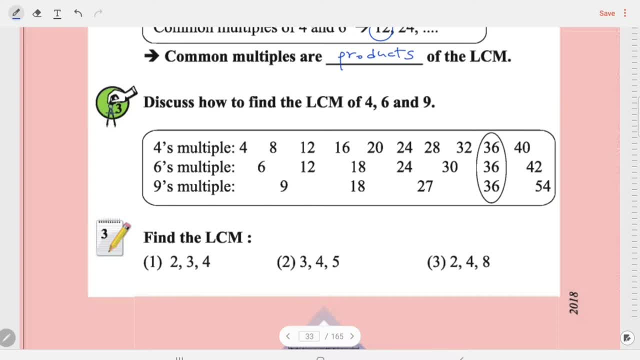 to see which number, which number is there among these? 3,, 4,, 6,, 9.. So 36 is the common number. you have to find that is the LCM right. see, 36 is the commonest. 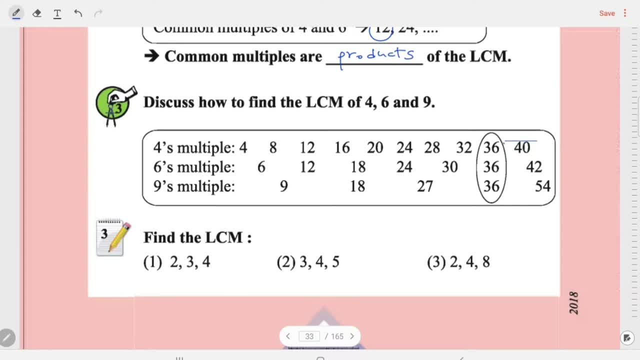 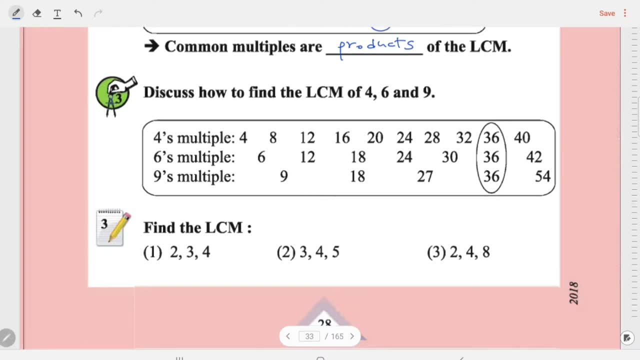 among them. so 36 is the LCM. ok, but this is quite arduous to find because takes plenty of time right? that's why I suggest you to use the method which we, which I taught you just now. what is the method? 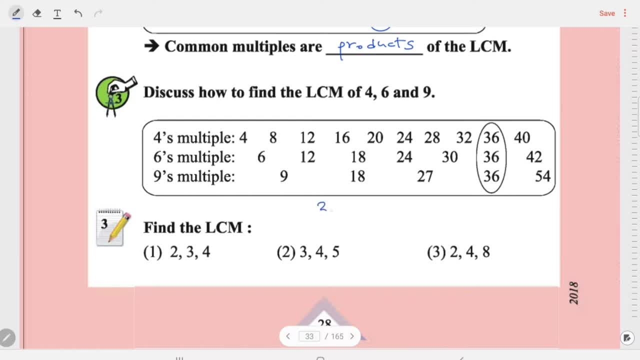 I am not going in the usual way Because it takes so much of time. 22 is a 1, 23,. 22 is a 4, ok, 33,. 22 is a 4, ok, so 2 x 2 x 3,, that is the LCM: 2 x 2 x 3,, 4 x 3, 12,. so 12 is the answer here. ok, 3, 4,. 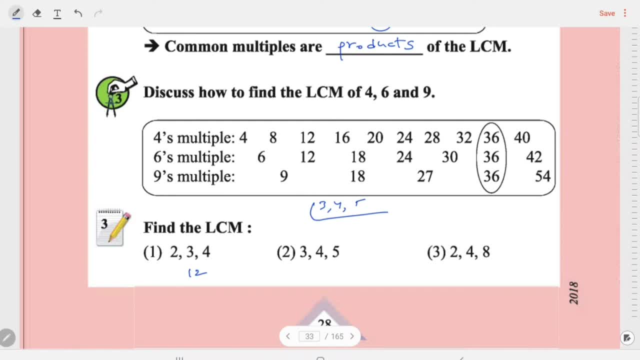 5,. again 3,, 4,, 5,. there are no common multiples. ok, So 4, 5 is a 20,. 20 is a 5,. ok, So 4, 5 is a 20,. 20 is a 5, ok. 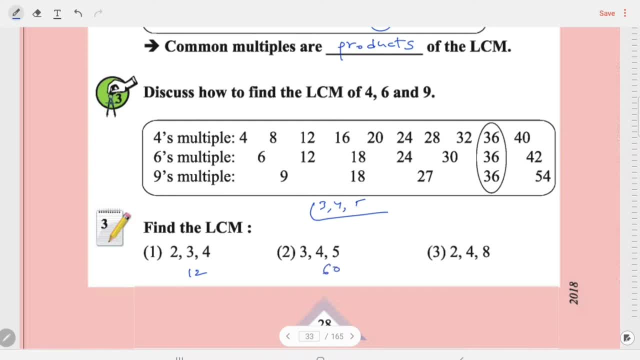 So 4, 5 is a 20,, 20 is a 5, ok, So 4, 5 is a 23,. 23 is a 60, that is the answer. When they are 4 primed numbers like 3,, 4,, 5, the product of the numbers gives you LCM. 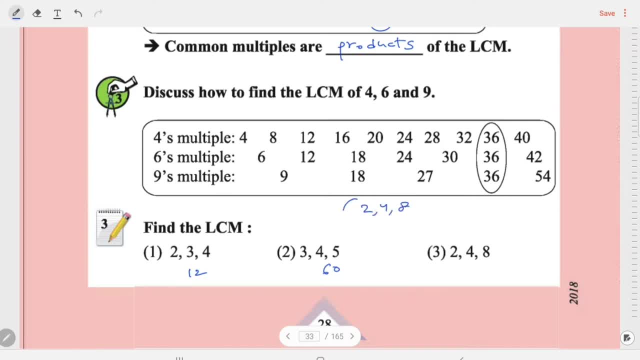 Now 2, 4, 8,. 2,, 4, 8,. you should start with 2, 2, 1 x 2, 2, 2 is a 4, 2,, 4, is a 8.. 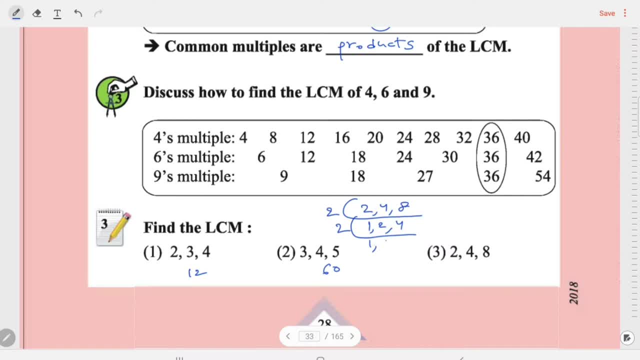 Again, you can proceed with 2.. 1 is 1, only 2, 2 is a 1, 2, 2 is a 4, 2 x 2 x 2 is how much 8.. 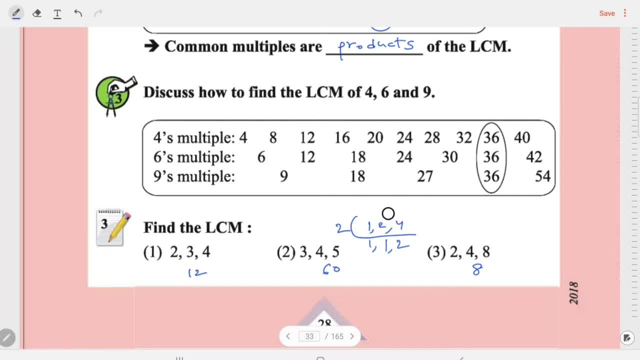 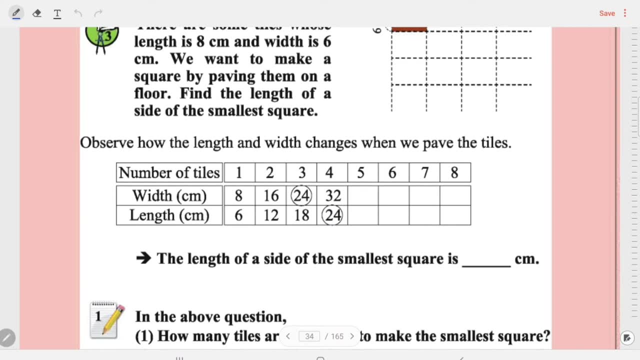 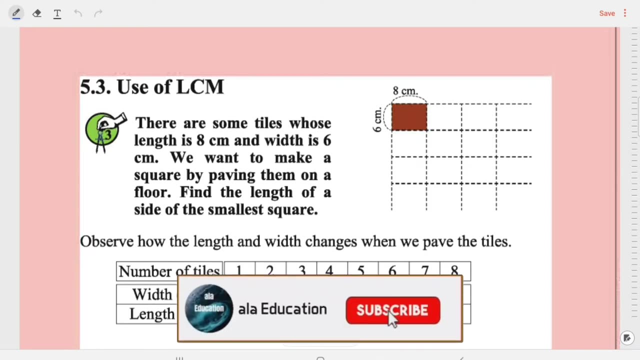 So the answer is going to be 8.. Ok, use of LCM. there are some tiles whose length is 8 cm and width is 6 cm. we want to make a square by paving them on a floor. find the length of the length of the side of a smallest square, then that. 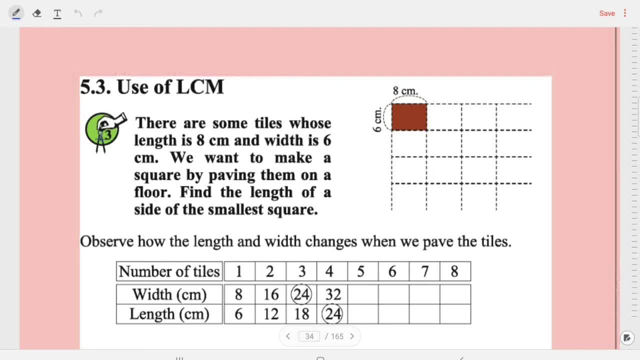 is going to be 6, right 6 into 6. observe how the length and width changes when we pave the tiles. number of tiles given: 8. when you take with the rate, then there's 6, like this: okay, when you, when you use two number of tails which will be doubled, length will be doubled three times. three times. 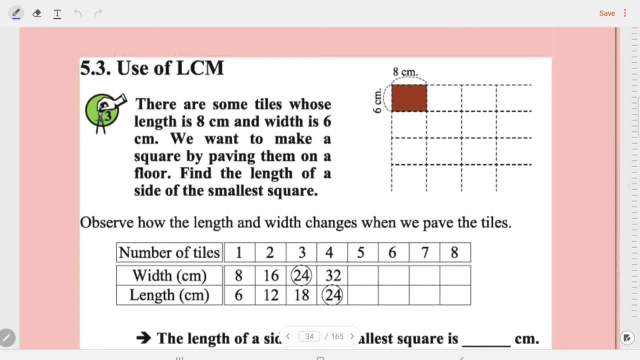 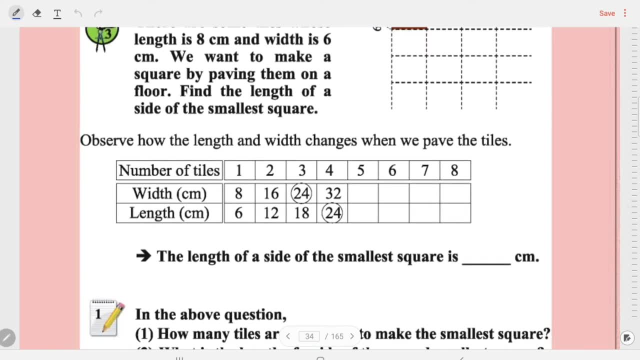 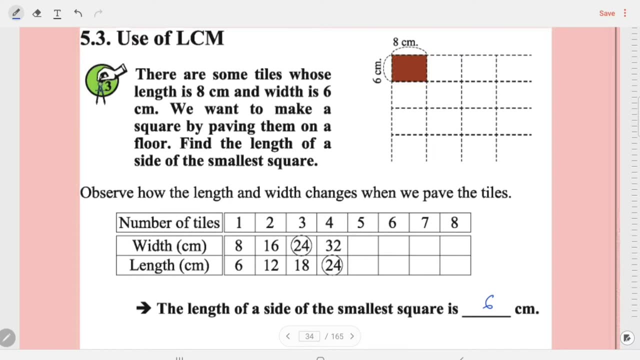 like that. okay, the length of a side of the smallest square is how much? 6 cm? oh, that must be a multiple of both right LCM. in this case you need to find the LCM that is 24 cm. it must cover both 8 and must be product of both 8 and 6, because it is not a perfect square, it is a. 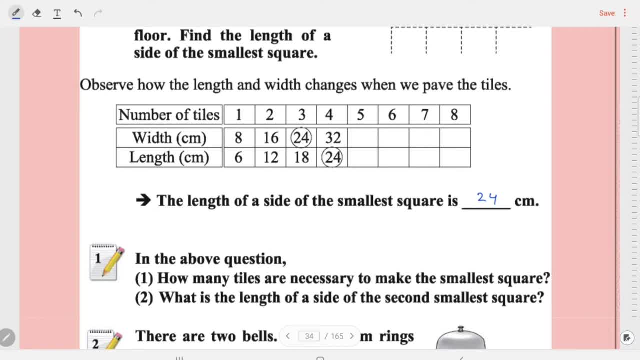 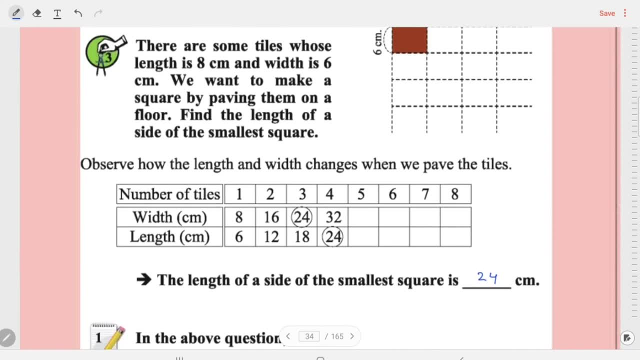 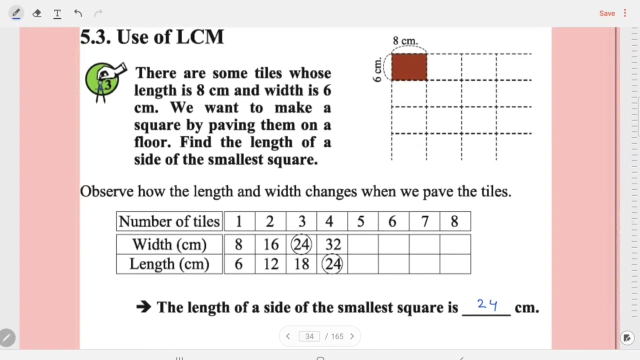 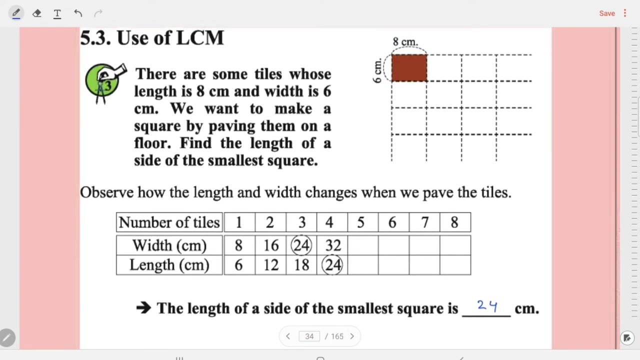 rectangle in the above questions. how many tiles are necessary to make the smallest square? how many tiles are necessary? four times right, far time. how many times the necessary make smallest square? the smallest square side is 24 cM golden. how many tiles are necessary to make smallest, if square? what is the length of thisры welcomed? 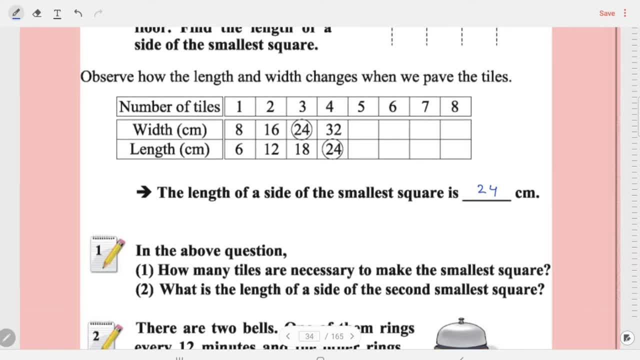 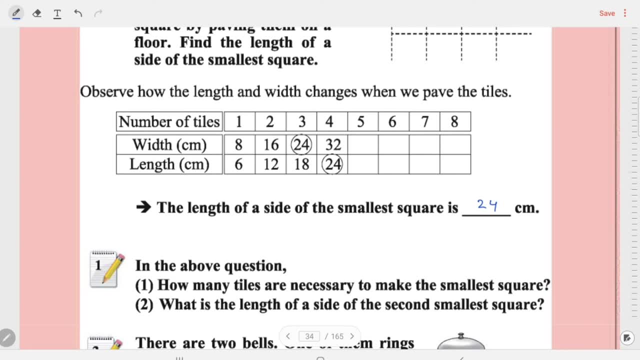 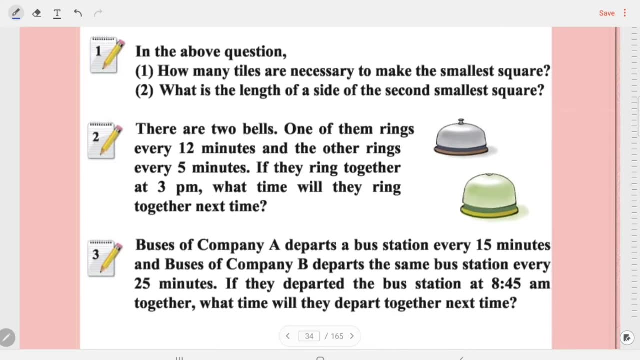 endto the direction of the length of the side of the bolt. how many times the length of the top of the second smallest square? didn't get it right. okay, forget about it. there are two bells. one of them rings every 12 minutes and other things in every five minutes. 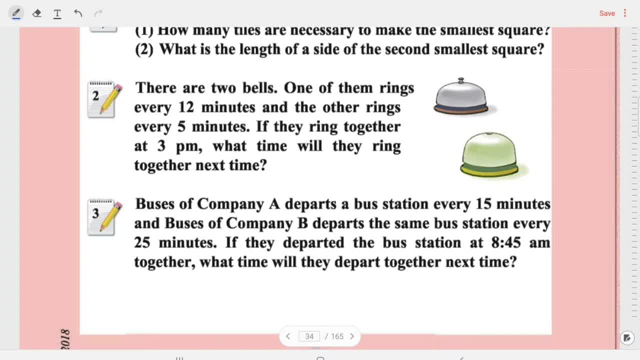 if they ring together at 3 pm, at what time will they ring together next time? this is also LCM problem. okay, again, 12 and 5. you can see they are co-prime. so 12 into 5 is LCM. that is nothing but tasty. my shoes don't year estimate. 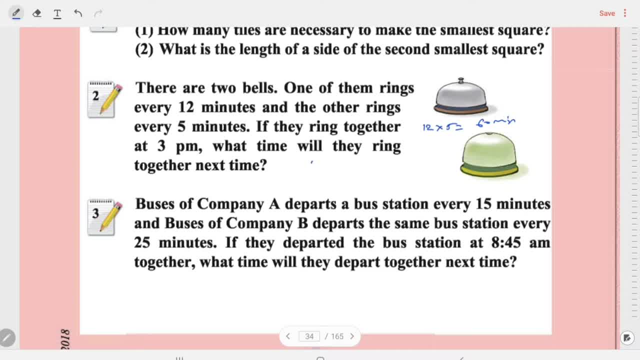 60 minutes means one over right, so at 4 pm again they will ring together, or you got the point right. one stuff: company a departs, say, bus station every 15 minutes and out of company P departs the same by station every 25 minutes, if they. 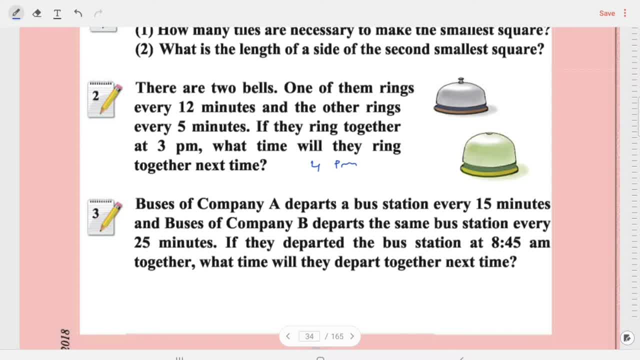 depend on the state, we get one hour left, they will leave to home. if they depend on the Beresford time, all time will be obviamente the same for somebody. if they depend on the Troy question, if they depend on the state็ covering less the bus station at 8: 45 am together, what time will the depart together next? 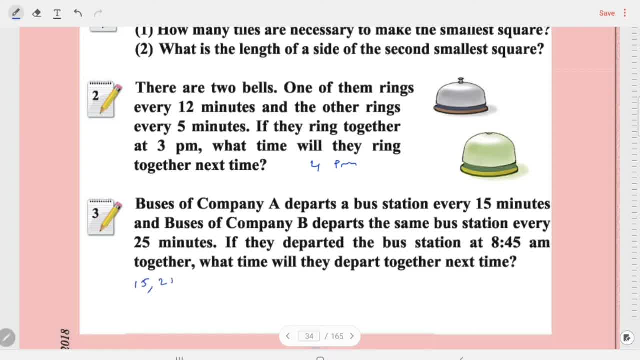 time again. this is LCM problem. 15, 25, 5, 3 0, 5 5 0, 25, 3 0, 75, 75 minutes is the LCM. you have to add this number to 8: 45. 75 minutes means 1 hour 15 minutes wait a. 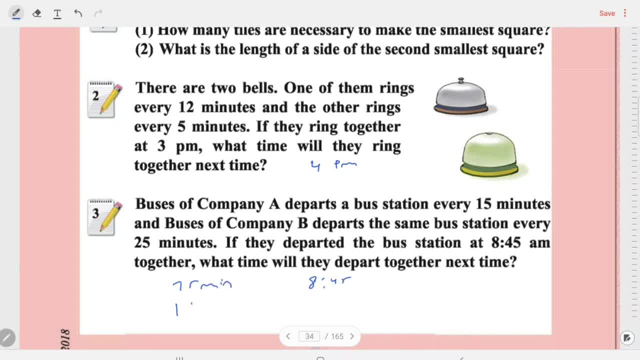 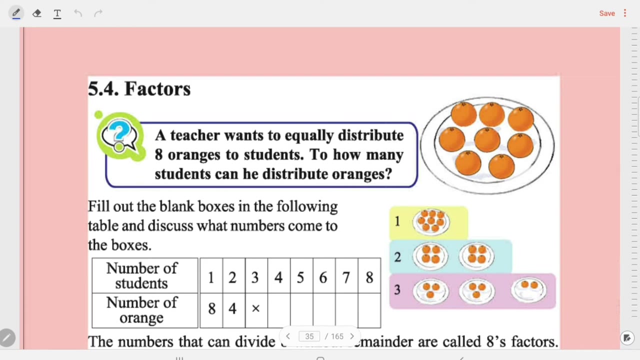 minute. let me write it clearly: 1 hour 15 minutes. you just add 1 hour 15 minutes, 8, 45, 10, so 10 am. they will depart together the next time. okay factors. the teacher wants to equally distribute eight oranges to students to. 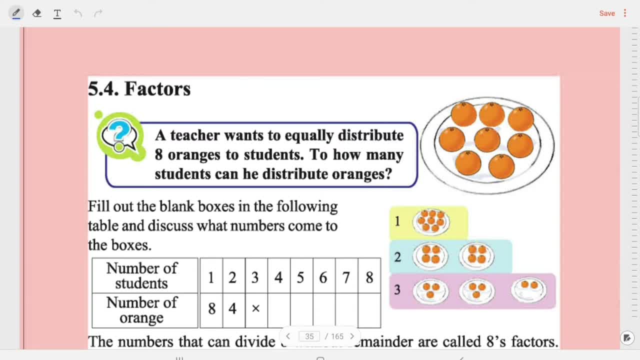 how many students can he distribute oranges at max? we can give it to eight. okay, if he is giving only one, you can give it to eight students. if he is distributing to two oranges, then we can give it to four members. okay. if he is distributing four, four and this, you can give it to two. 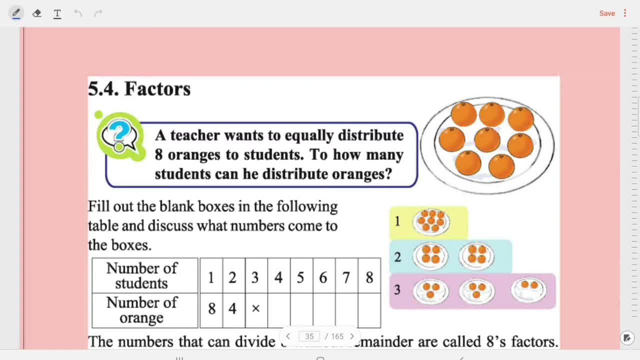 students only qualité или done with it. and if he's distributing- all eight are in this- to one fellow, then it will go to only one. suppose and fill out the blank boxes in the following table and discuss what numbers come to the boxes. number of students: one means. 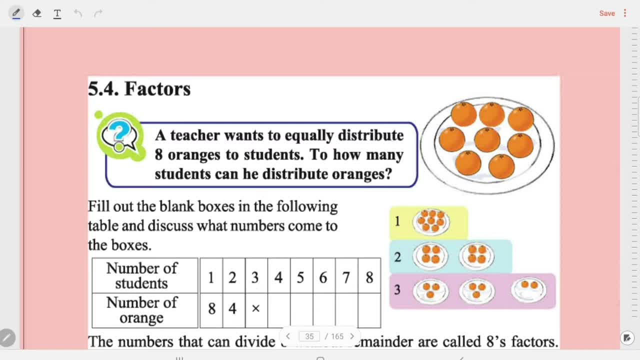 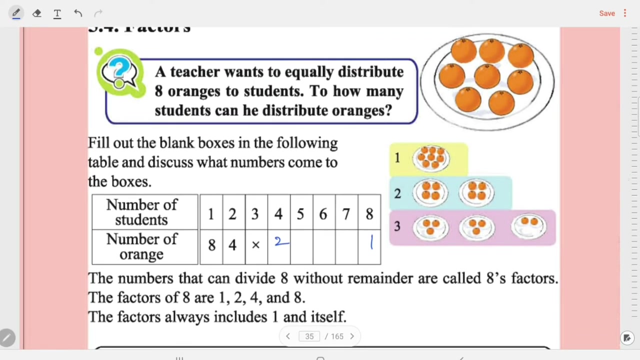 eight are just to only one. two minutes for three minutes. know you cannot do the ship it because three is not a factor fate. four is fine, you can give it to two, it to 2 students: 5,, 6,, 7,, no 8 is 1.. So the numbers that can divide 8 without remainder. are called factors of 8.. The factors of 8 are 1,, 2,, 4,, 8.. The factors always include 1 itself, 1 and itself, The number itself and 1, both are the factors. N's factor is: 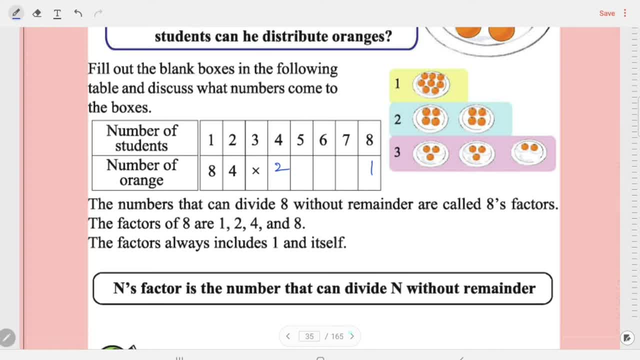 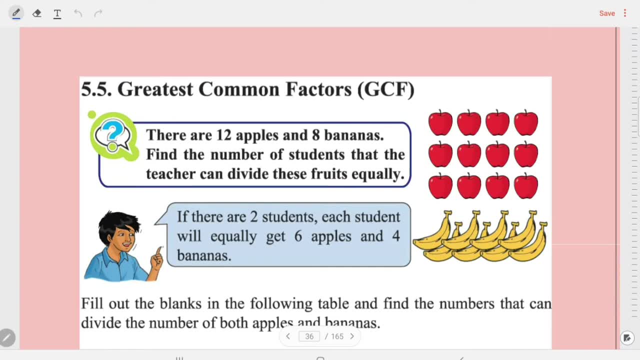 the number that can divide N without any remainder. Greatest count factor. What is GCF? Greatest count factor? There are 12 apples and 8 bananas. See here in the picture These are 8 bananas. These are 1, 2, 3, 4, 1, 2, 3, 4 into 3, 12.. 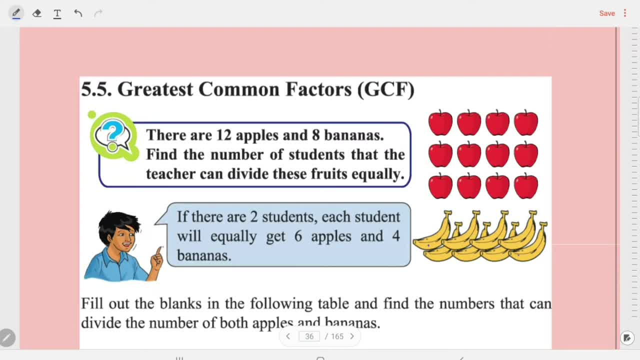 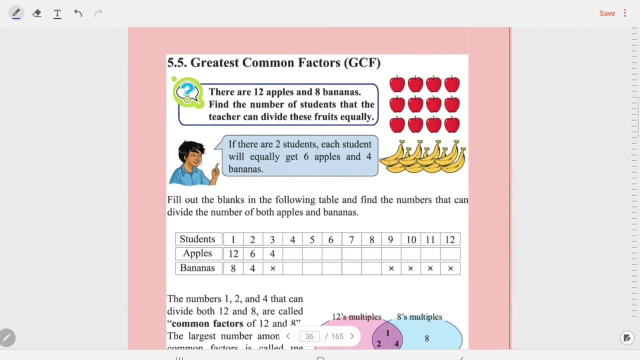 That the teacher can divide these fruits equally. Find the number of students that the teacher can divide these fruits equally. If there are 2 students, each student will equally get 6 apples and 4 bananas. This is the greatest count factor problem. Oh wait. 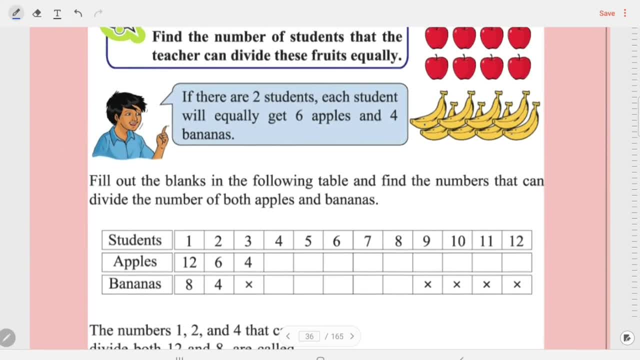 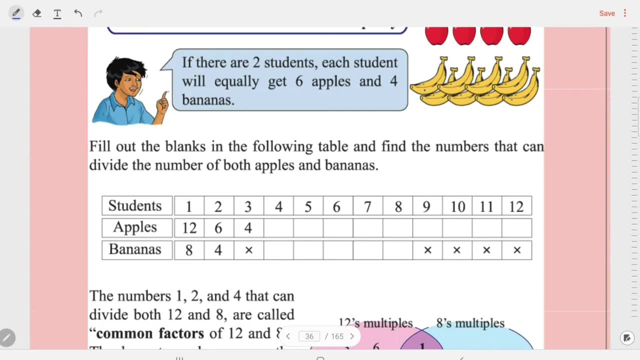 a minute. All right, Fill out the blanks in the following table and find the numbers that can divide the number of both apples and bananas. One student means 12 apples: he will get 8 bananas. Two students means 6 apples and 4 bananas. 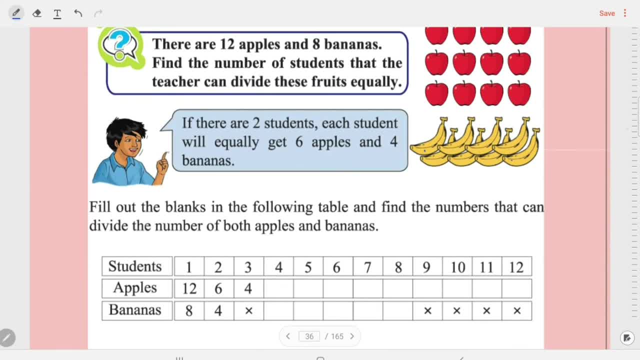 One student means 8 bananas. Look at the number in the table. One student means 12 apples and 4 bananas. Two students gives 5 bananas. One student gives 16 bananas. One student gives 8 bananas. Two students gives 16 bananas. 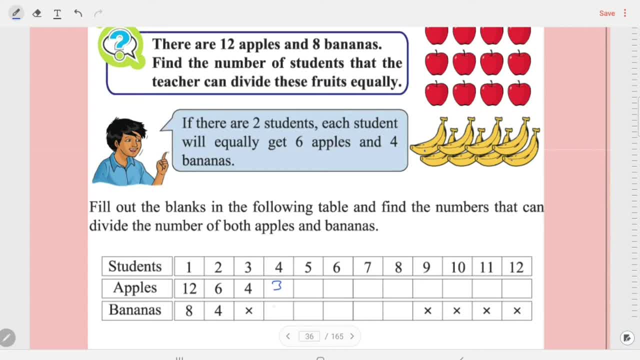 Two students gives 18 bananas. Two students gives 18 bananas, Three students gets 17 bananas. Three students gives 30 Biscigns time 45 seconds. So there are 15 bananas. city inventors already have 15.. 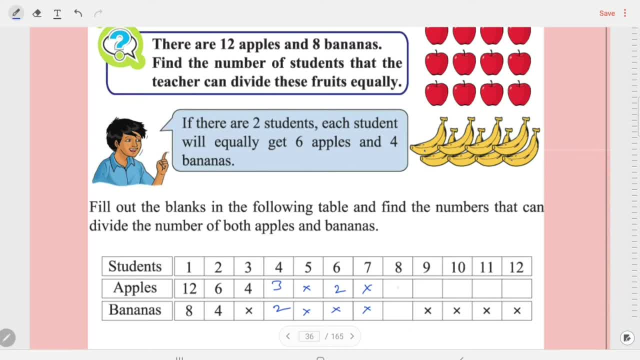 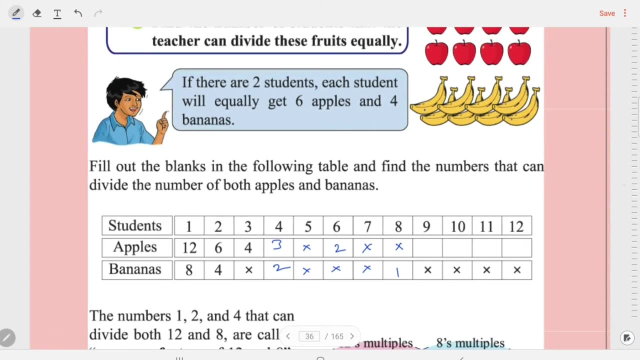 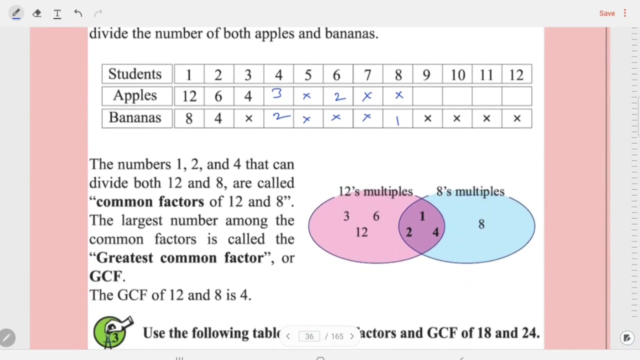 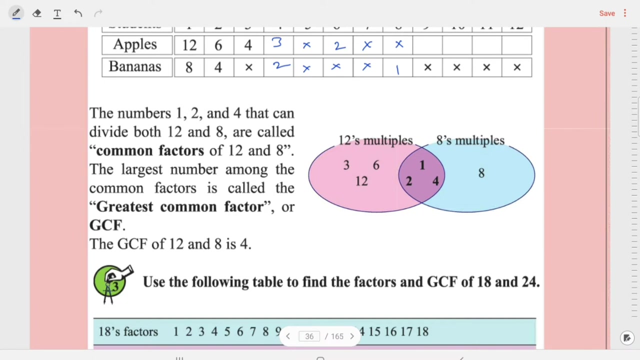 filled in the blank. both are not the connectors. 8. this is not a connector. okay, that's it. the numbers are 1, 2 and 4 that can divide both. 12 and yes, they wait. 12 and 8 are called count factors of 12 and 8, the largest number. 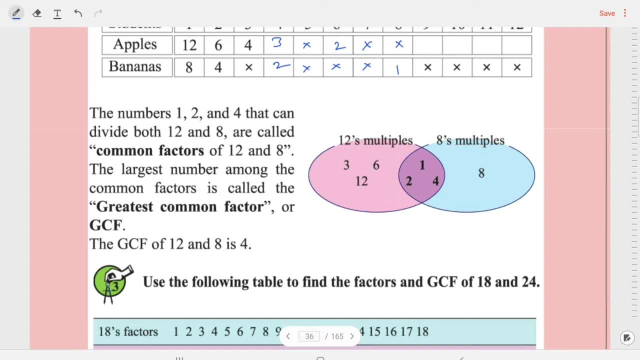 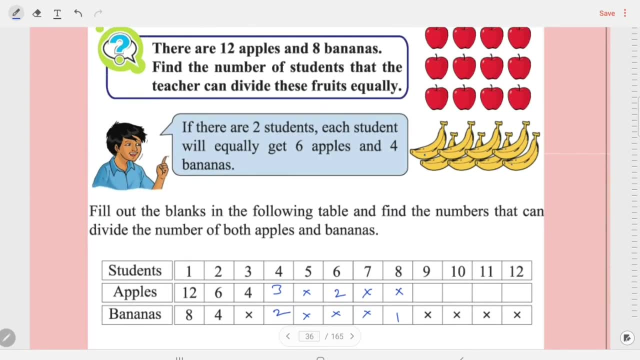 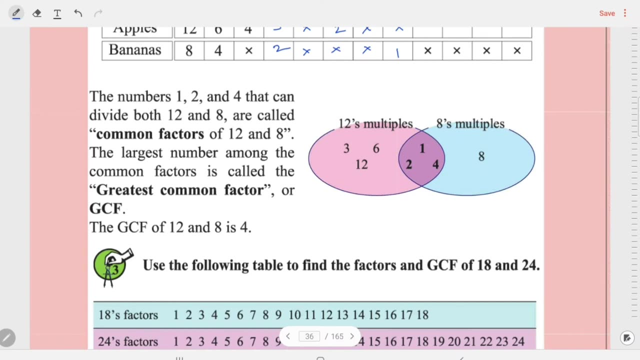 among the count factors is called greatest count factor, GCF. okay, in this case it is 4. okay, so GCF. here is the 4. okay, you have to find the count factors. okay, greatest among the count factor is GCF. okay, all right, or use the following table to find the. 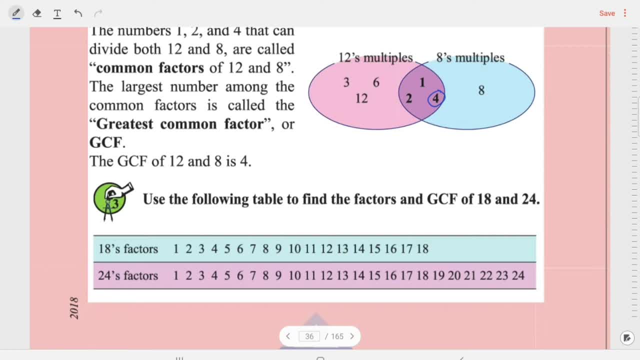 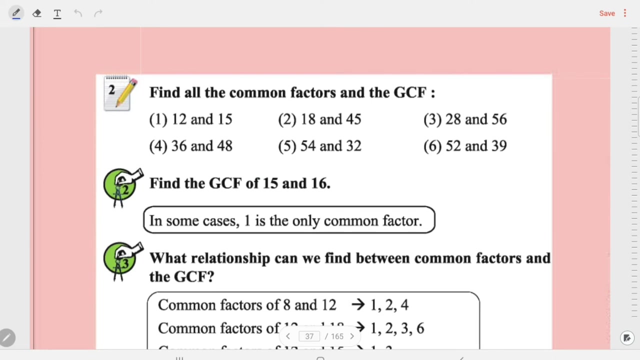 factors and GCF of 18 and 24. 18 factors are what? 18, 18, 2 to 36. okay, like that you have to proceed. forget about it. we'll see another example: find all the count factors and the GCF. I will do only one problem: 12 and 15. let's see 12- what. 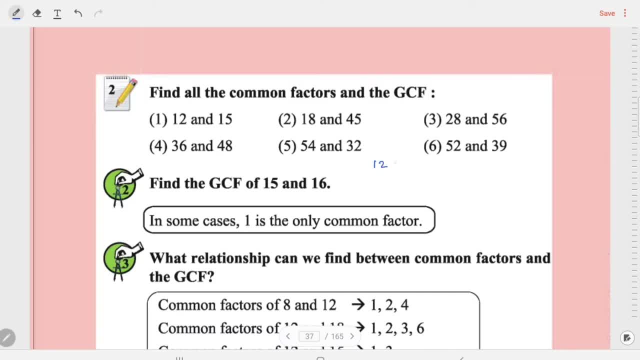 is the count factors of 12 and 15. 12 factors are 12, 24, 36. oh sorry, 2, 3, 4 and tall 15 factors were 3. wait a minute. 15 factors are 3, 4 and 12. oh, wait a minute. 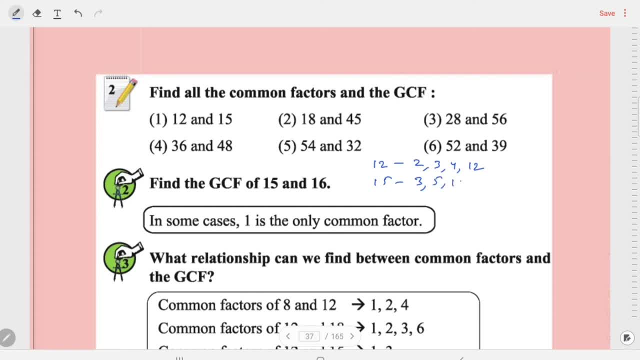 3,, 5 and 15. also, I haven't written 1.. 1 is also a factor, of course. What is the greatest count factor? In this case, it is 3.. GCF is 3.. These are the factors of these two numbers. 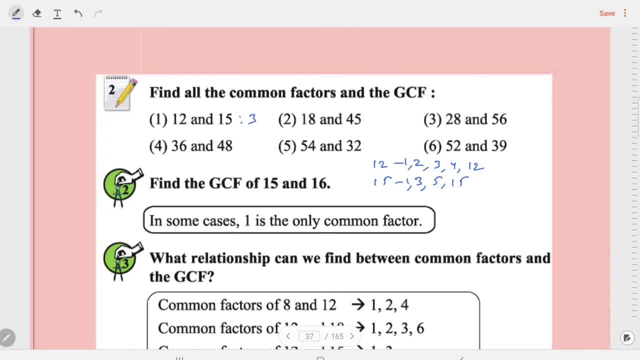 and among them the greatest factor is 3. Find the GCF of 15 and 16.. In some cases, 1 is the only count factor, 15 and 16.. Yes, In that case, when they are co-prime, 1 is the only. 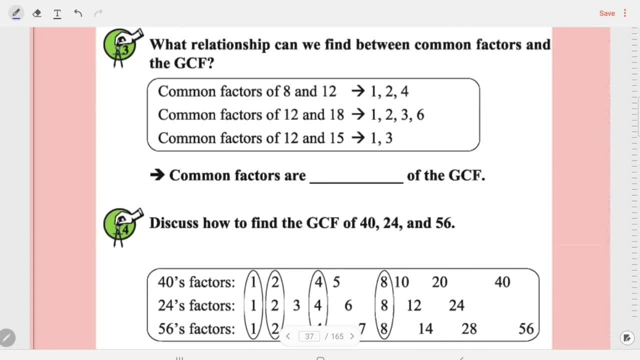 count factor. So GCF is 1.. What relationship can we find between count factors and the GCF? What is the relation? Let's see: Count factors of 8 and 12 are 1,, 2, 4. Count factors. 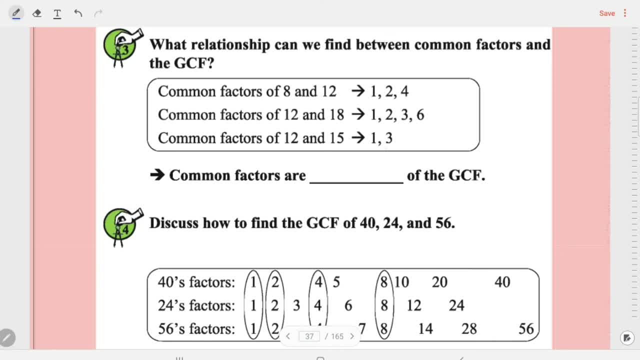 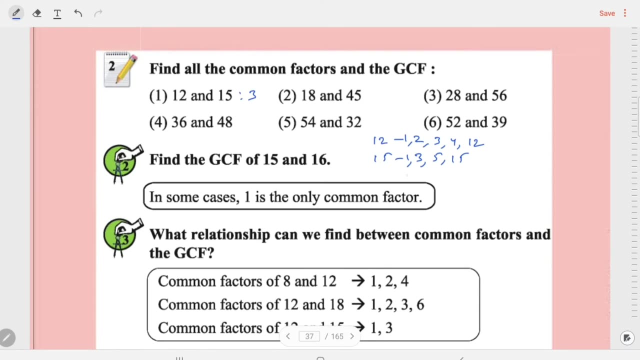 of 12 and 18 are 1,, 2,, 3, 6.. Count factors of 12 and 15 is 1, 3.. Count factors are dash of the GCF, Multiples of the GCF In this case. Is that so? 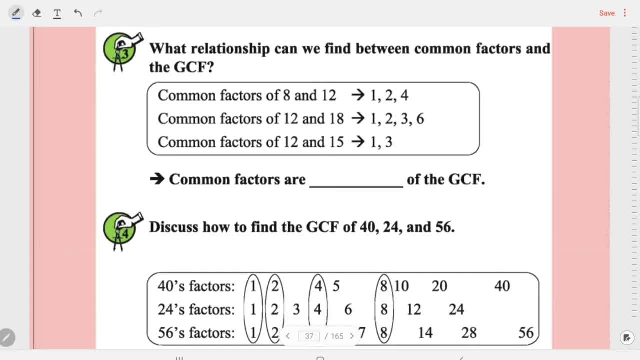 Discuss how to find GCF of 40,, 24 and 56.. 40's factors, These are 40's factors, These are 24's factors And these are 56 factors. Okay, See, these common factors are circled. 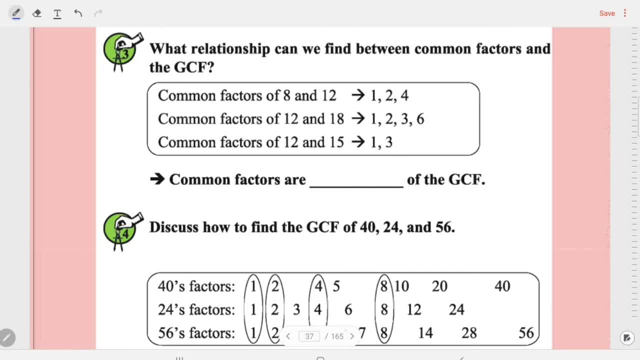 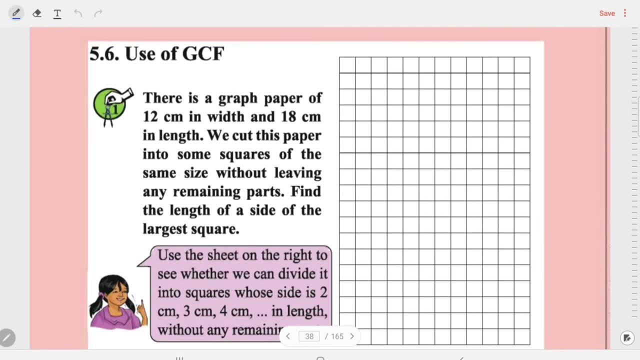 here, The greatest among them is 8.. Right, So answer is 8.. There is a graph paper of 12cm in width and 18cm in length. We cut this paper into some squares of the same size without leaving any remaining parts. Find the length of the length. 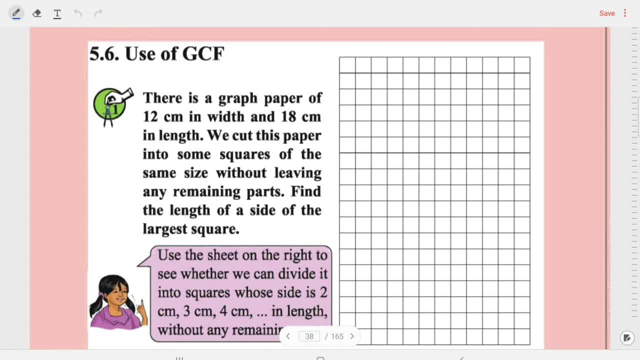 of a side of the largest square. Use the sheet on the right to see whether we can divide it into squares whose side is 2 cm for cm in length without any remainder. You can also do something likeomos commercial. You can write in your a congestionlights section. 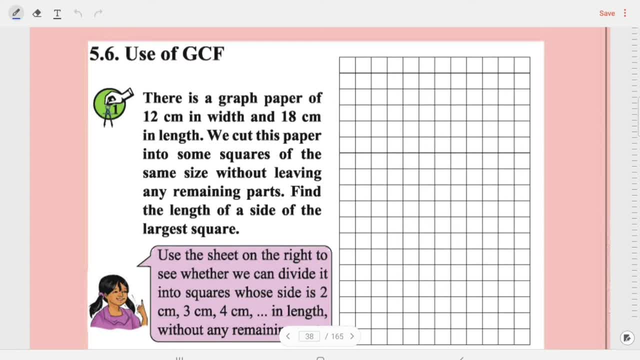 Well, Write a information line for a a US bank, anda for a chronological souventu Crisis: Elimination Problems. Dividing it next: Kr birdie decrease is 1. When the without any remaining parts: right, so you need to find gcf1 in this situation. 12 and 18: how to find. 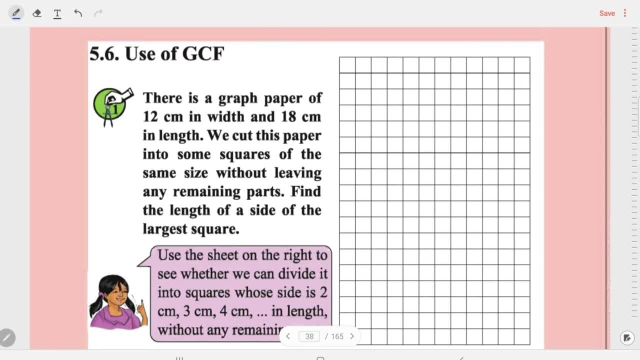 gcm. take a small number, okay, divide the small number with the larger number, 12, 1j, 12. here you get 6, 6, twos of 12. so 6 is the answer, 6 is the gcf in this case. so what is the answer? 6 centimeter. 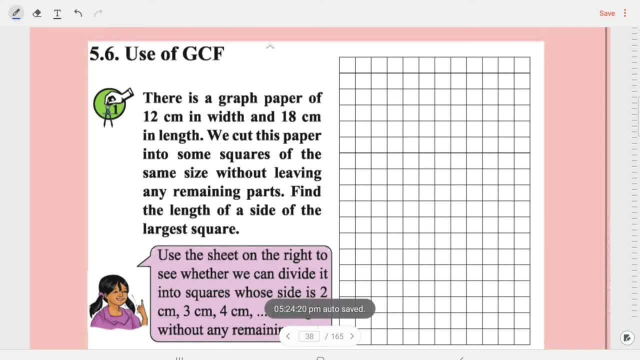 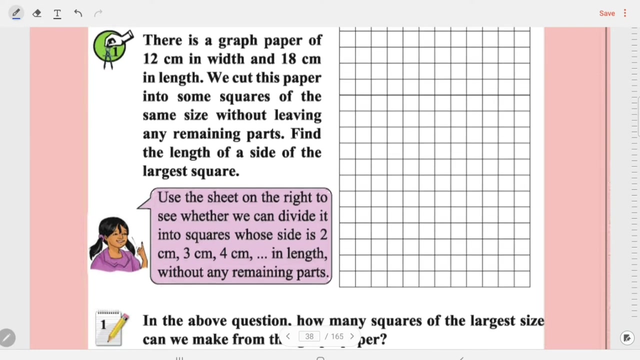 okay, so 12 into 18, divided by six into six, this is 6. 3 is your 12, six three is your 18, that is nine. so nothing will remain here. in this case, you can use only nine squares of 6 cm size. okay, in the above. 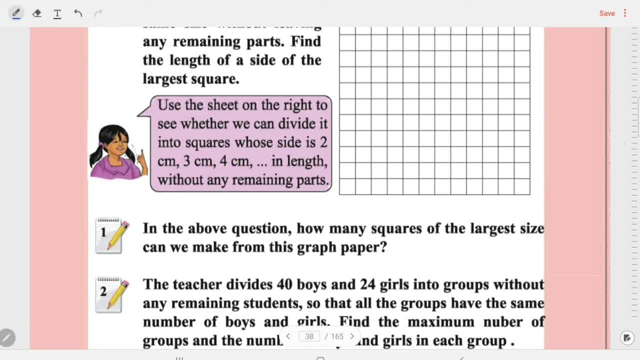 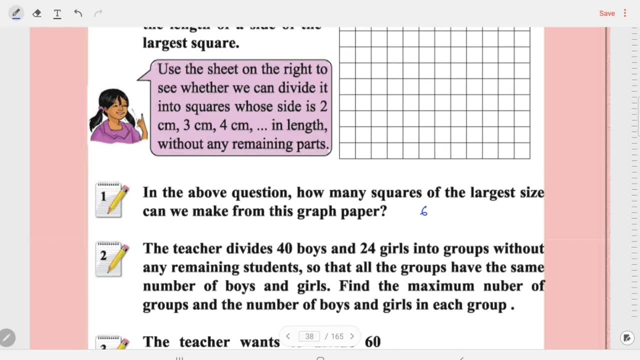 question: how many squares of the largest state can we make from this graph paper? just now, we got it right: nine, okay. the teacher divides 40 boys and 24 girls into groups without any remaining students, so that all the groups have the same number of boys and 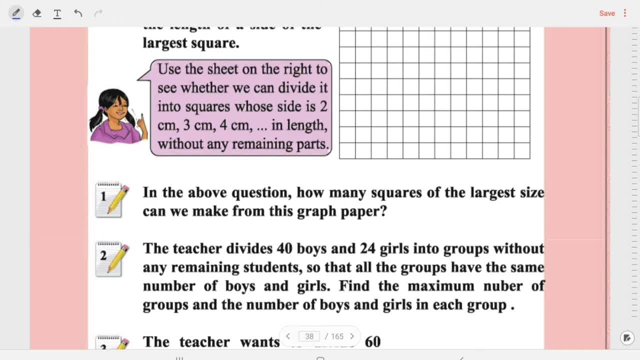 girls find the maximum number of groups. that, and the number of boys and girls in each group: 40, 24. proceed like this: 24, 1 to 24. now this is 16, i guess. yes, 16, 16, 16, 8 will come 8 to the 16, so 8 is the answer okay. 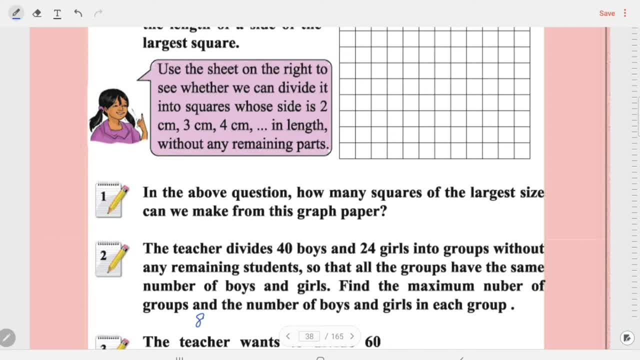 8 is the gcf. okay, what is the number of groups then? eight boys, eight girls in the first group. second group: again eight boys, eight girls. third group: eight boys, eight girls. only you can form three groups. okay, find the maximum number of groups and the number of boys and girls in each group. 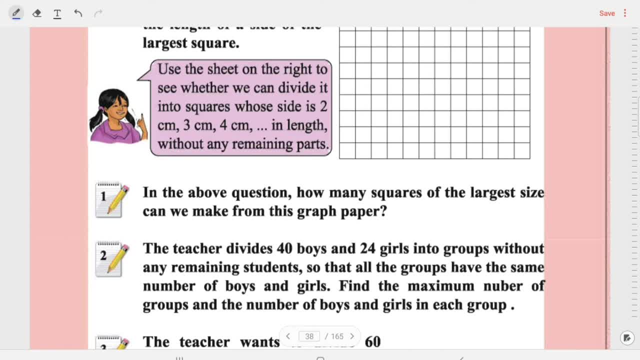 so if you want to find the maximum number of groups, you can make 24 groups as well. okay with. by using only one boy and one girl in each group, you can go up to 24 groups, okay. anyway, that is not going to be solved by gcm. the teacher wants to divide system. 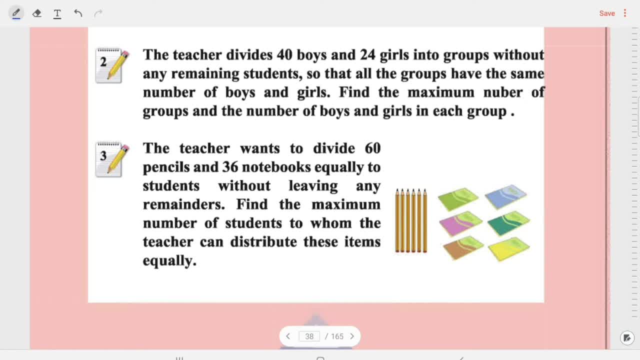 so who gives term them like 19, three brothers. you will have one boy, one girl, which is eighteen, and one and one girl. or change g8 kolej. now, if one of the group is open, when the school 적led with it by clicking one down, 12 and 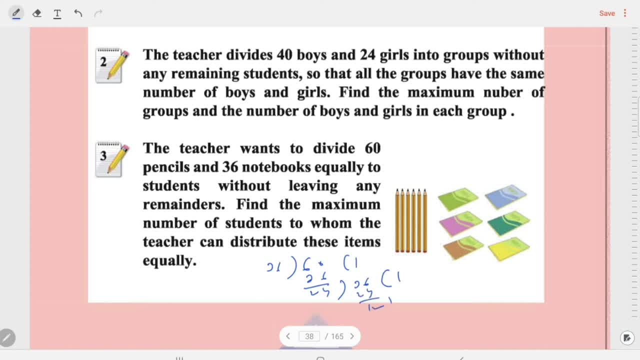 Maximum созд. one is correct: 36,. two is not correct. one is rare: is 12, 12, 224, so answer is going to be 12,. all right, so teacher can distribute them equally among 12 students. okay, without without having any remainder. 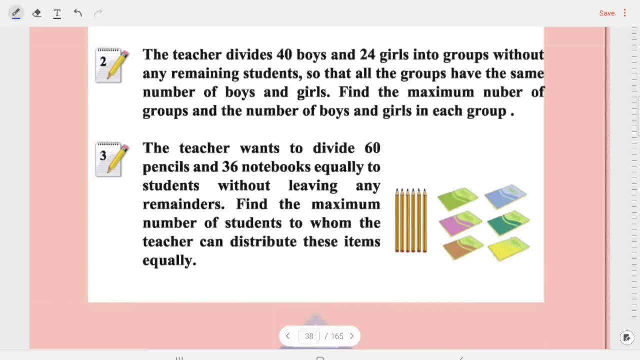 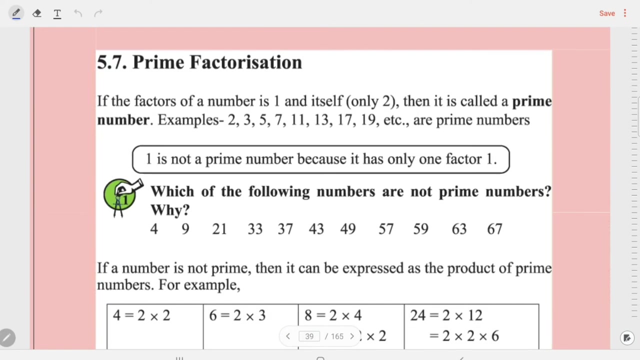 okay, 40,, 24,. what is the GCM? okay, forget about that. there, the there, you need maximum number of twos. okay, okay, calm down, calm down. prime factorization: if the factors of a number is 1 and itself, then it is called prime number. 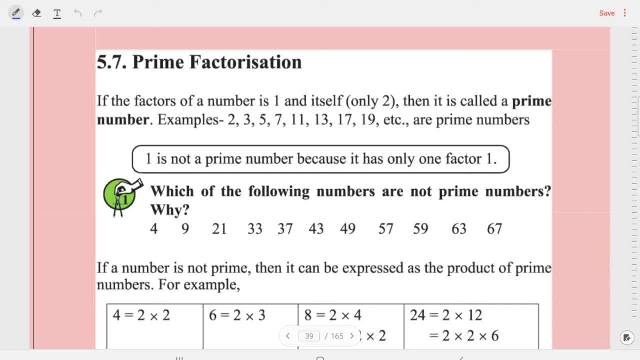 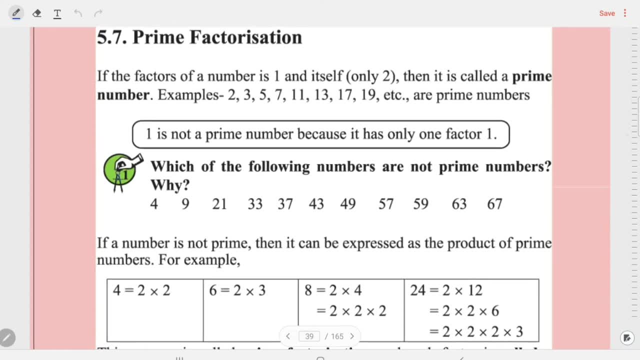 examples of prime numbers are 2,, 3,, 5,, 7,, 11,, 13,, 17,, 19,. 1 is not a prime number because it has only one factor. which of the following numbers are not prime numbers, and why? because they have. 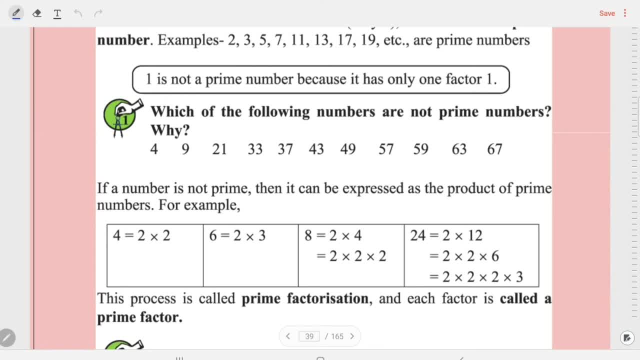 if they have factors other than the number itself and 1, then they are not prime. like 4, it has factor of 2, 9 also, this is also not prime. 9 is factor of 3,. here 3 and 7 are the factors other than the number itself and 1,. 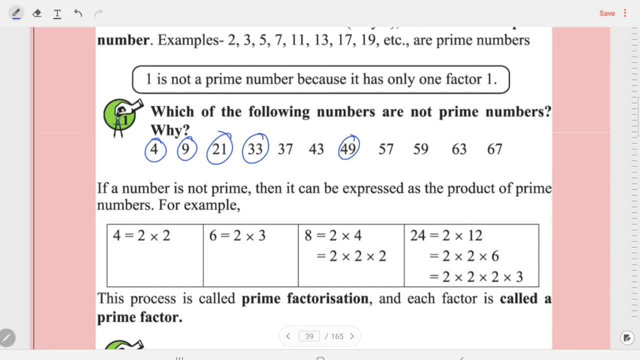 here also. this is 49,, 33 also. 11 is a factor, 3 is a factor. 49,, 7 is a factor. 57,, 3 is a factor. okay, 63,, 3 is a factor. 7,, 7, 7 is a factor. 9 is a factor. if a number is not prime, then it will be. 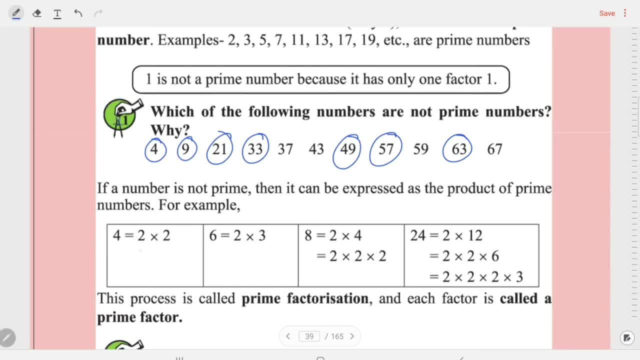 expressed as a product of prime numbers, like example 4, 2 x 2,, 6, 2 x 3,, 8, 2 x 4,- okay, 2 x 2 x 2,. only in terms of prime numbers you can express that factorization is called prime factorization. 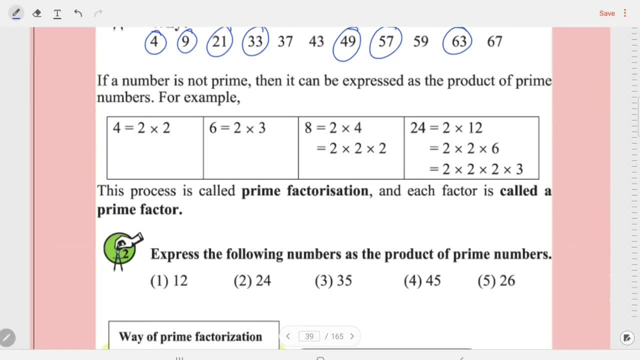 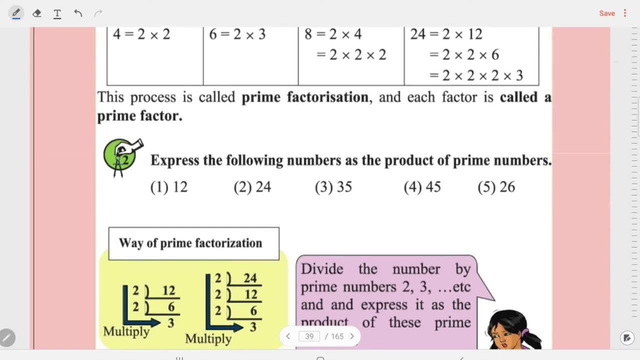 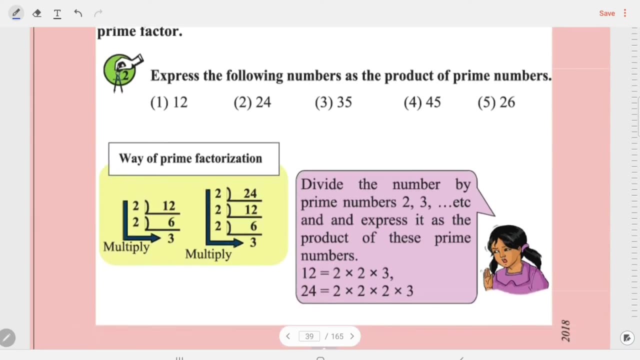 okay, process of this, process of writing a number. okay, as the product of primes is called prime factorization. okay, and each factor is called prime factor. I took, I will take only one example here to illustrate: okay, all right, 12. 12 means 2 into 6, 6 is 2 into 3, this is 1, 24. also, they 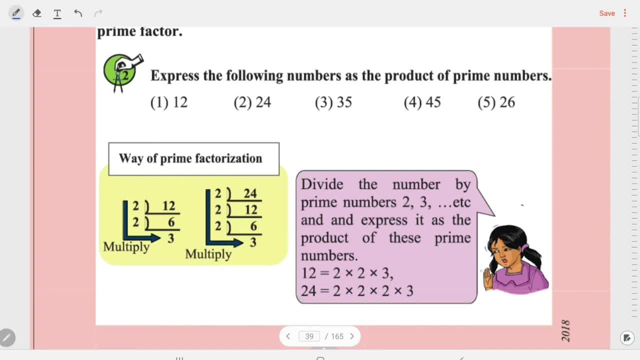 did it okay. 35, let me do it for 35. 5 into 7. that's it. whatever. you won't get many. this is 5 into 7. so we have prime factorization like this: 2 into 6, 2 into 3, 2 into 2 into 3, okay. 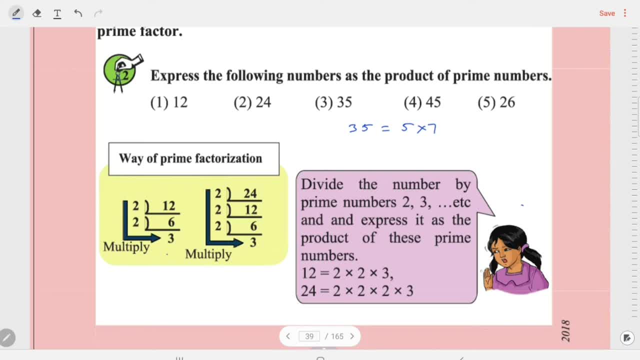 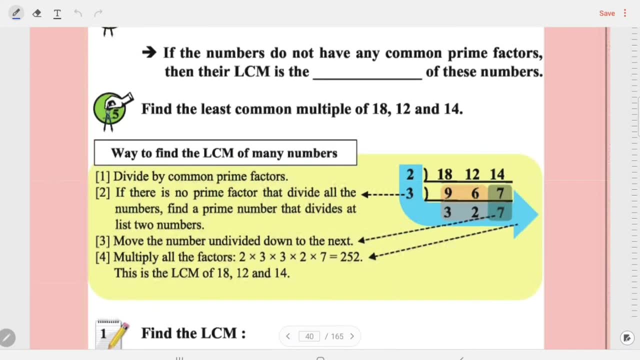 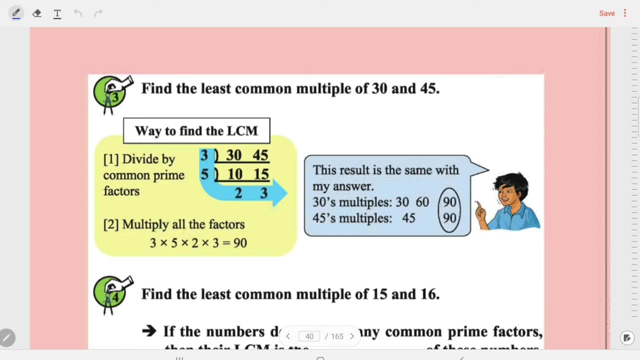 like that. you can proceed to find the prime factors. find the least common multiple of 30 and 45. they will become prime factors. like I told you earlier, multiply all the factors, see first. you can proceed with. you can also proceed with 2, it is the okay. your 3 is not a factor, so proceed with. 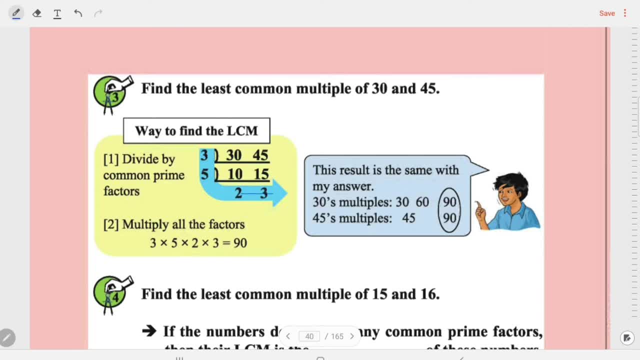 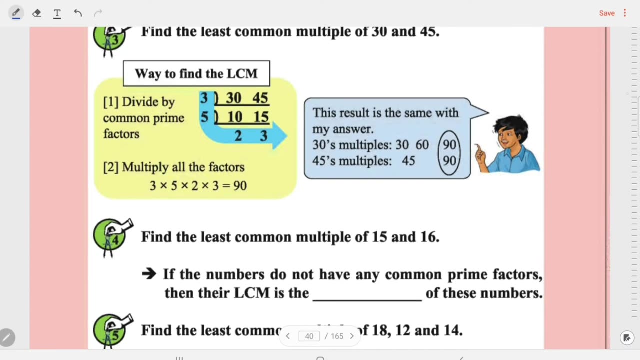 3, 3, 10 to 30. 3, 15 is a 45, 5, 2 is a 10, 3 is a 15. multiply them together: 5 into 3, 15, 15, 2 is a 30, 33 is a 90. so 90 is the LCM least common multiple. okay, 15 and 16, these, these two are co-prime. 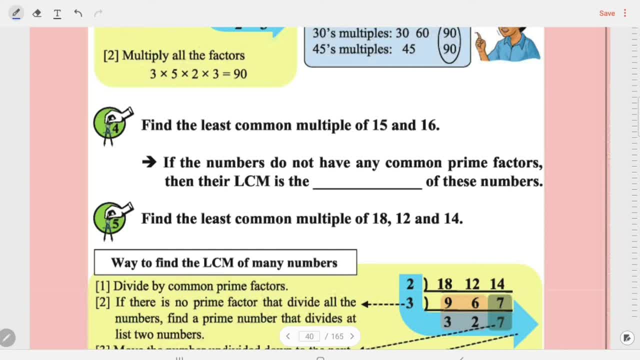 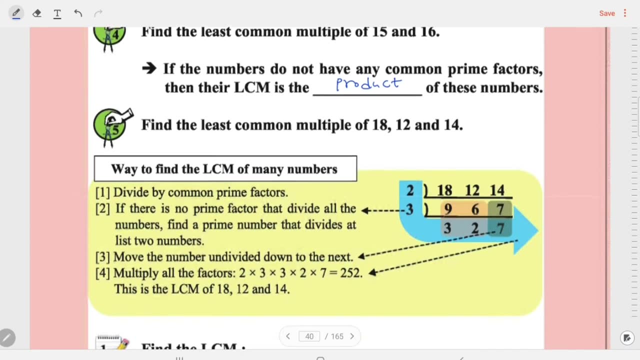 factors. okay, so product of the numbers. if the numbers do not have any common prime factors, then their LCM is the product of these two numbers. product of these numbers? okay, there are two or three, how many numbers they may be, that must be product, find the least. 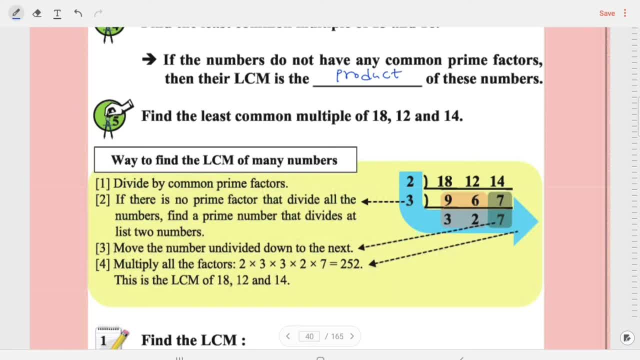 common multiple of 18, 12 and 14 like this: 2, 9, 18, 2, 6, 12, 2, 7, 0, 4. again 3, 3, 3 0, 9, 3, 2 0, 6. that's it all our times. right now, you multiply 2 into 2 into 2, 2 square into 3. 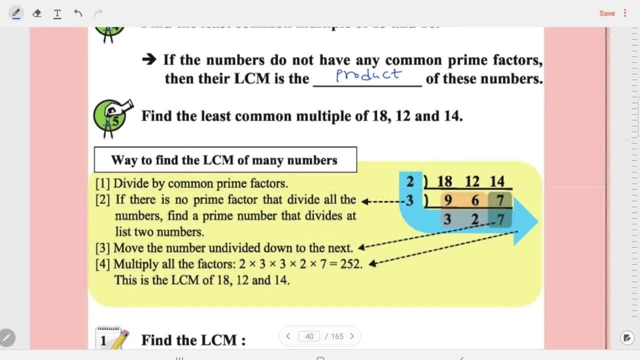 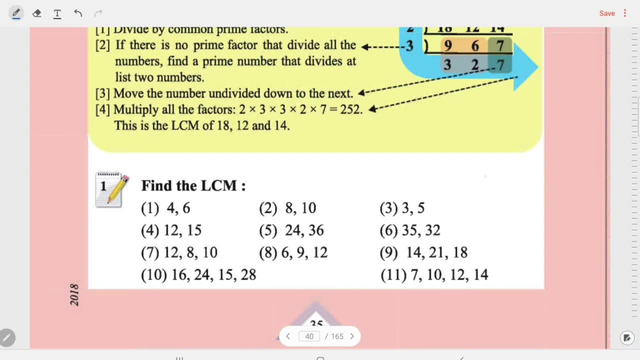 square into 7. so answer is 252. that is the LCM of those numbers. let me do it for 8 and 24 and 36. okay, 2, 12, 0, 24, 2, 18, 0, 36, 2, 6, 0, 12, 2, 9, 0, 18. again 3, 3, 2 0, 6, 3, 3, 0, 9. so 2 into 2, into 2, into 3 into 3, that is 8. 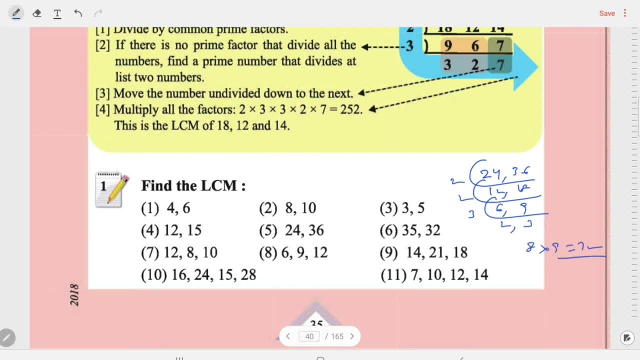 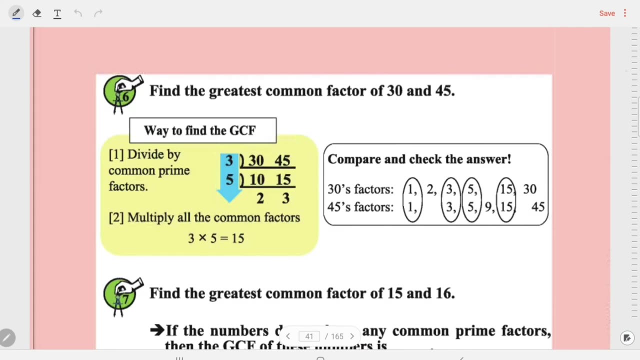 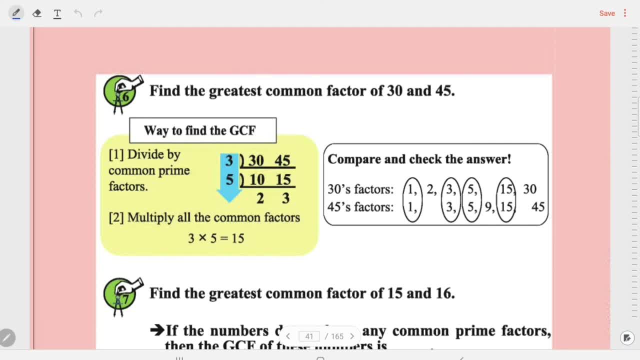 find the greatest count factor. again, you can also find GCF by means of prime factorization. okay, so divide the common prime factors like this: 30 and 45. okay, multiply all the common factors. What are the count factors? 3 into 3 and 5 in this case. That is the greatest count factor. 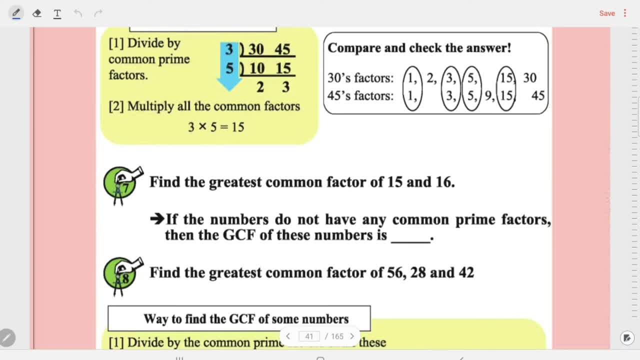 This is the easiest method. Now, what is the greatest count factor of 15 and 16?? That is, the numbers do not have any count prime factors, then the GCF of the numbers is the product of the numbers. The numbers do not have any count prime factors, then GCF of these numbers. 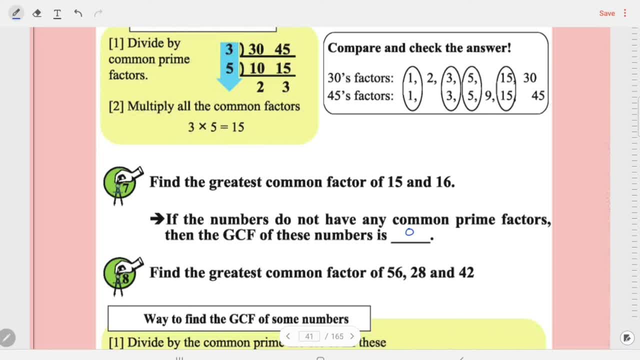 is 0.. There is no count factor. Find the greatest count factor of 56,, 28 and 42.. Again, proceed by the method which we discussed earlier, prime factorization method. 56,, 28,, 42, like this: 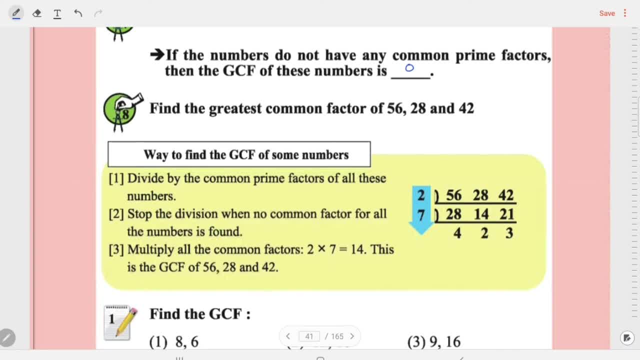 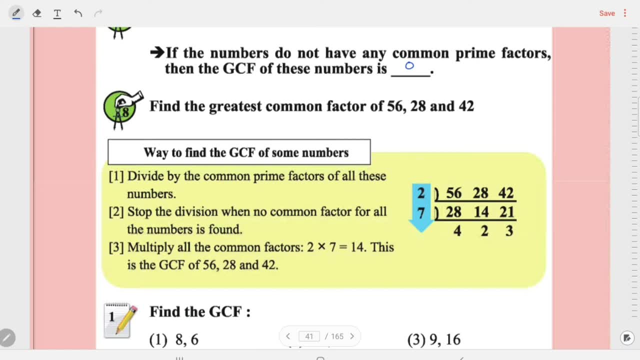 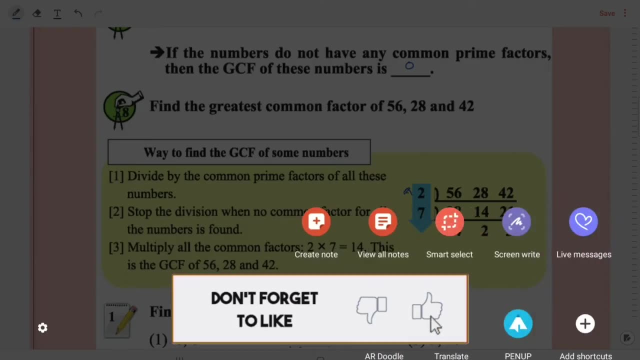 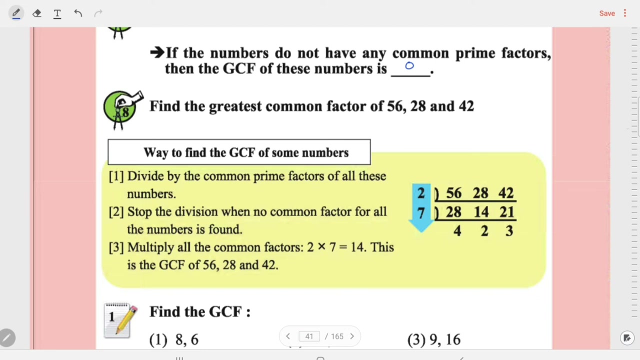 228 is 0,, 214 is 0,, 221 is 0,, 74 is 0,, 72 is 0,, 73 is 0.. So 2 into 7, that is it. Thus, that must be the factor of all the numbers right. So 2 into 7,. 14 is the GCF, Let me. 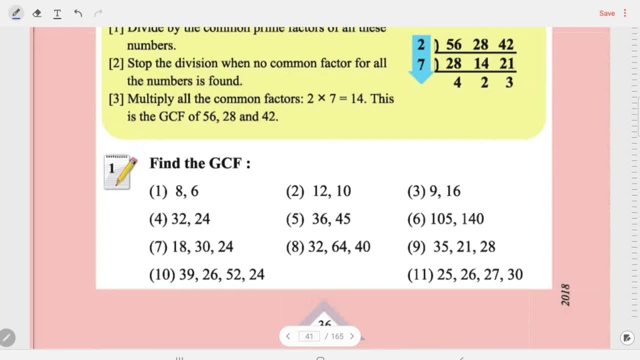 do it for 32,, 64, 40.. 32,, 64,, 42 is a factor right. 260 is 0,, 232 is 0,, 220 is 0, again 2, 28 is 0, 260 is 0,, 210 is 0, again 2, 24 is 0, 28 is 0, 25 is 0.. That is it, So this. 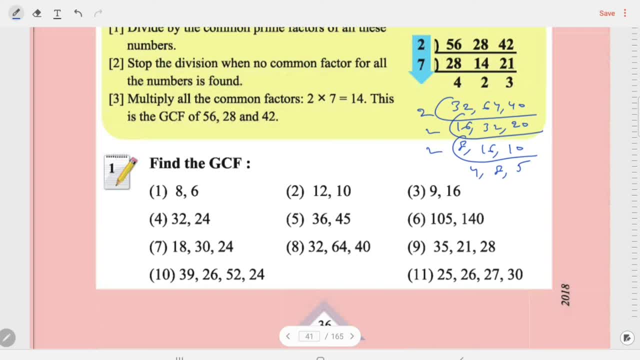 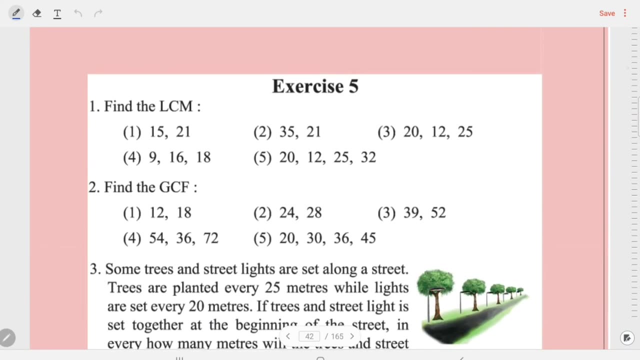 is the村. so 2 x 2 x 2 is the answer. that is 8. so here the answer is 8. ok, next xh5 is waiting for us find the lcm. ok, let me do it. let me do 20, 12, 25, 32. the last problem: 2 x, 10 x, 2 x, 6 x, 2 x, 16 x. 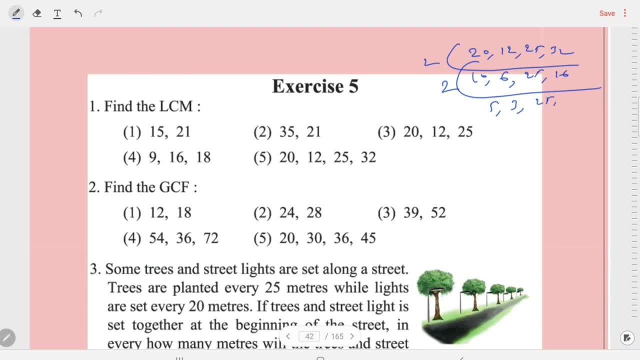 again: 2 x, 5 x, 2 x, 3 x, 2, 8. okay, now proceed with 5, 5, 1, 3, 5, 5, 8. now multiply: 4 x, 3 x, 25 x, 8, 25 x, 200, 200 x, 12, 0, 0, 2, 4, 0, 0. 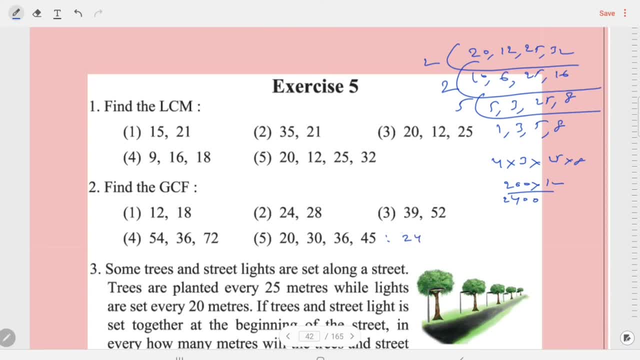 so that is the answer for this. oh wait, a minute, not here here. 2, 4, 0, 0. okay, find the gcf greatest count factor. okay, let me do it this one: 20, 30, 36, 45. is there a factor which is common among everything? no, 3, no, 5, also no, straight away no, so the count. 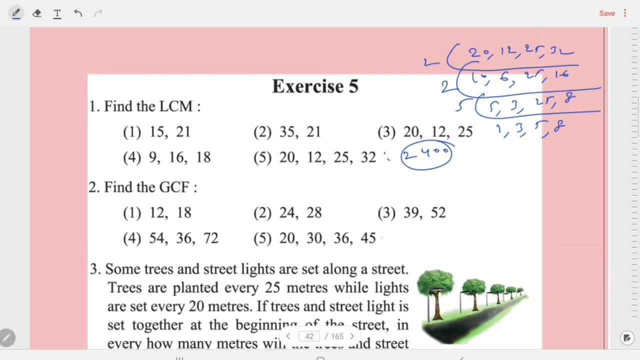 greatest count factor is zero. when there are no count factors, answer is going to be zero. okay, let me do 24, 28, 2, 12, 2, 14. again two, six, yeah, two, seven. yeah. so two into two is four. that is the answer, okay. 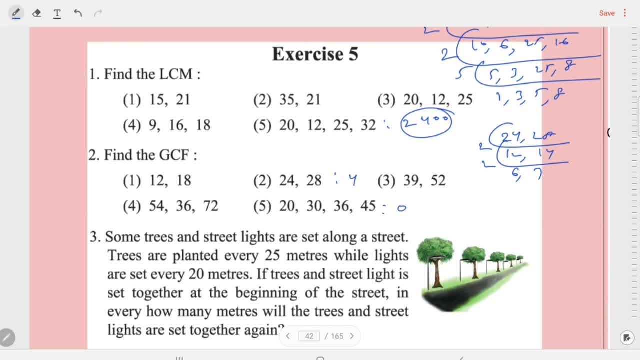 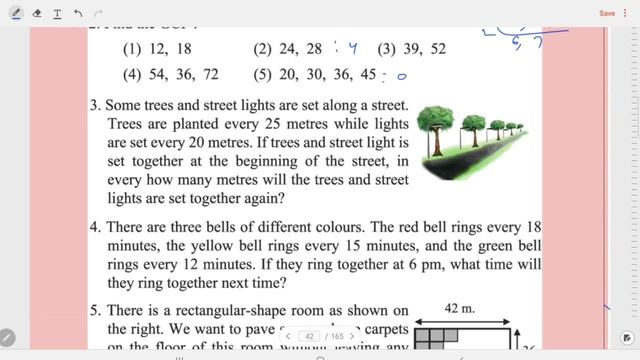 some trees, oh wait, a minute, some trees, uh, and streetlots are set along the street. trees are planted every 25 meters, so i lights are set every 20 meters. if trees and street lights instead are together at the beginning of the street, in every How many meters will the trees and street lights are set together again? 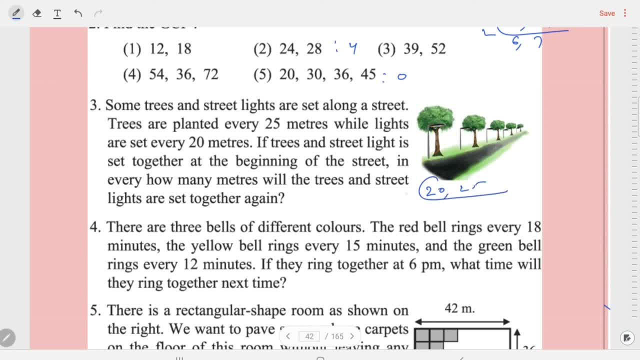 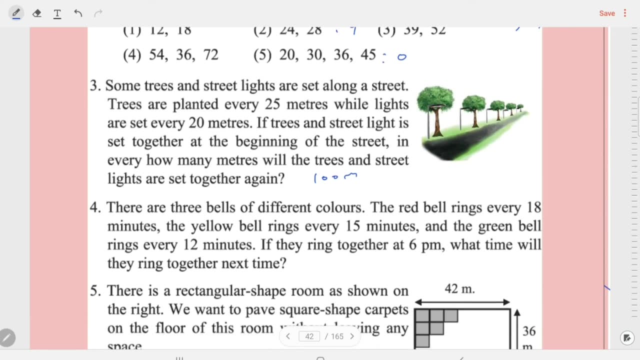 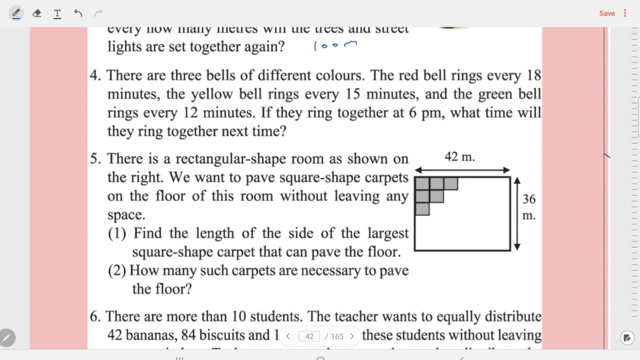 That is the LCM of 20 and 25, 5.4 J, 5.5 J, so 100.. So in every 100 meters they will coincide. There are three bells of different colors: The red bell rings every 18 minutes, yellow bell rings every 15 minutes and the green 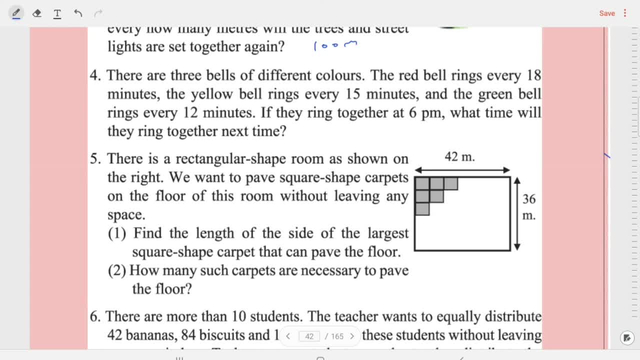 bell rings every 12 minutes. If they ring together at 6 PM, at what time will they ring together next time? This is also LCM problem. 18,, 15, and 12,, 29 J, 215 J, 26 J, 33 J, 35 J, 32 J. that's it. 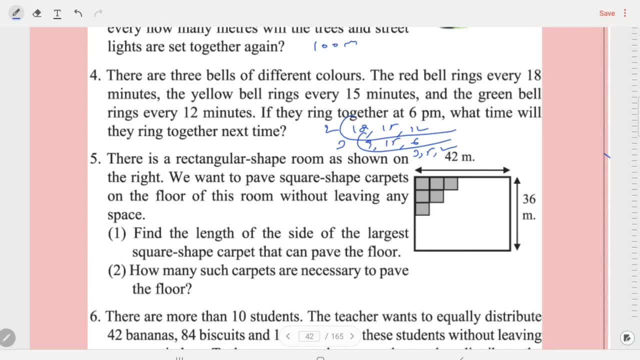 right. So the time is 6 J, 6, 10 J 60, 63 J 180.. So after 180 minutes. 180 minutes means 3 hours, so at 9 PM, Is that correct again? 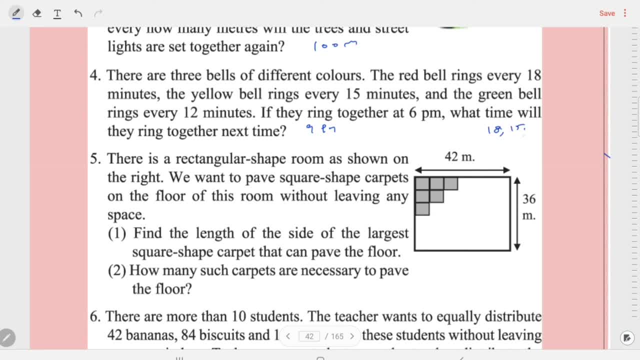 Can I let? let me check it again: 18, 15,, 12, 29 J 215, J, 26, J, 33, J, 33, J, 33 J. 3, 3 is a 3, 5 is a 3, 2 is a right right. 2, 3 is a 6, 10, 6 into 10,, 60,. yes, 3, 15. 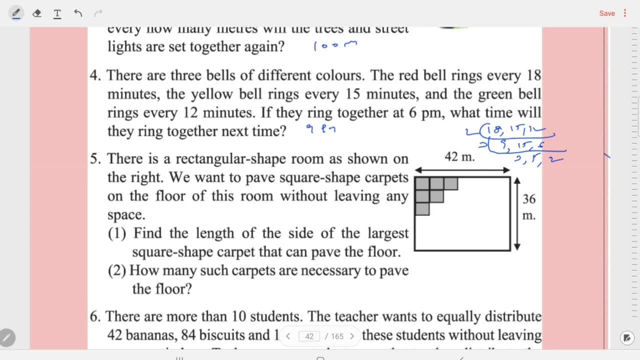 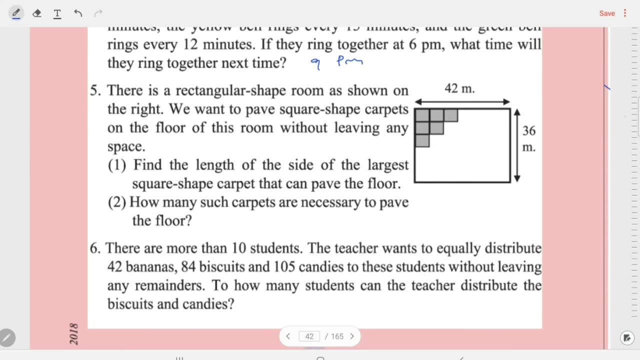 into 10 to 30,, 32 is a 60,, 63 is a 180, 180 minutes only. that is, after 3 hours, that is, at 9 pm. if there is a rectangle shape room as shown in figure on the right, we want. 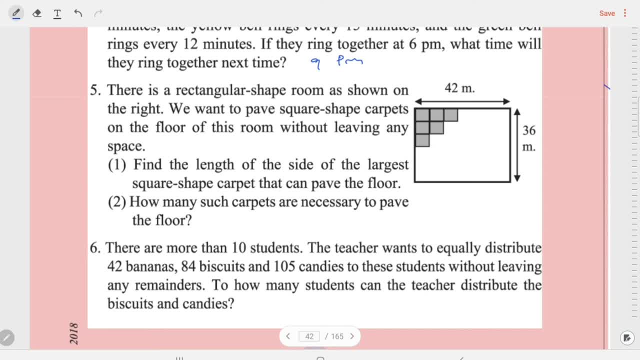 to pave square shaped carpets of the floor of the room without leaving any space. find the length of the side of the largest square shaped carpet that can pave the floor, so that must be GCF of 36 and 42.. Okay, 2, 18 is a, 2, 21 is a. again, 3, 6 is a, 3, 7 is a, so 2 into 3, 6,, so in this case that 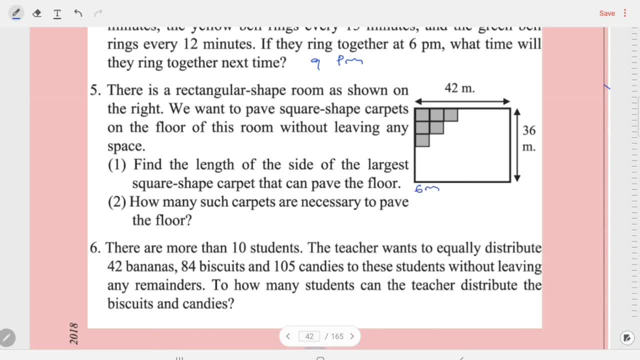 is 6 meters is the answer. how many such carpets are necessary to pave the floor? 42 into 36, divided by 6 into 6, okay, 6, 7 is a 6, 6 is a. So you might be needing 42 such squares. 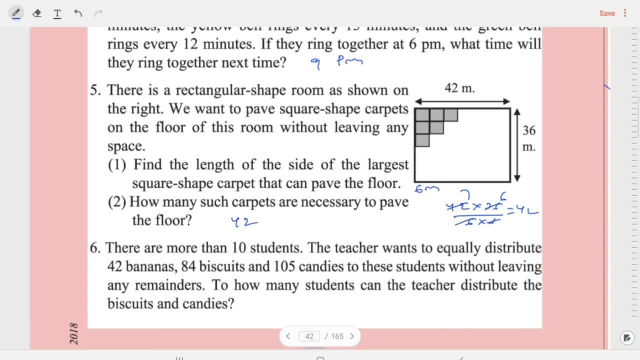 There are more than 10 students. the teacher wants to equally distribute 42 bananas, 84 biscuits and 105 candies to the students, without leaving any. a reminder to how many students can teacher distribute the biscuits and candies? okay, 42,, 84, 105. 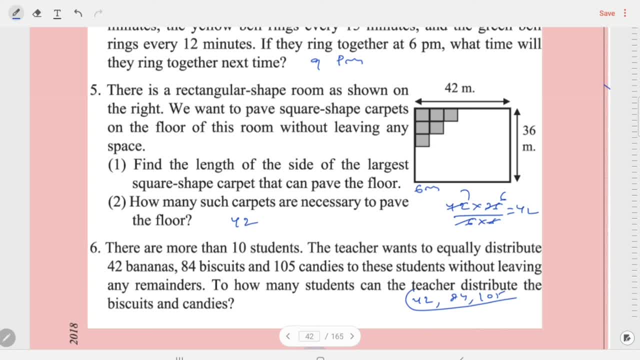 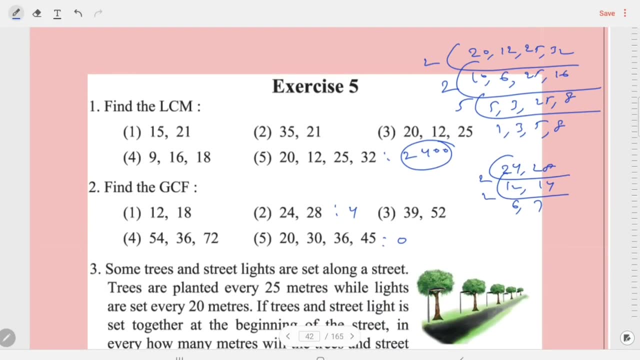 Okay. Hmm, That is the change here. Now you can also change them to嗯: Also in the course exam. I don't have perfect time criteria. no, you is, I don't have perfect time, but okay. 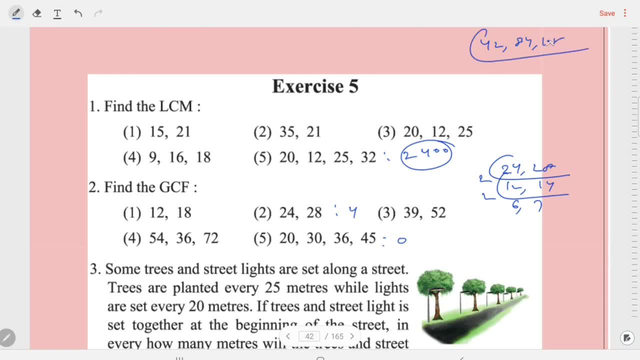 Another topic that you can consider easy to remember in aுhC is the use of perfect forget everything's for fake red. Let us break just a just a very Just this in: Okay, Okay, All right, dem unrealizezzo. So fine, insteadaletters there what we do. 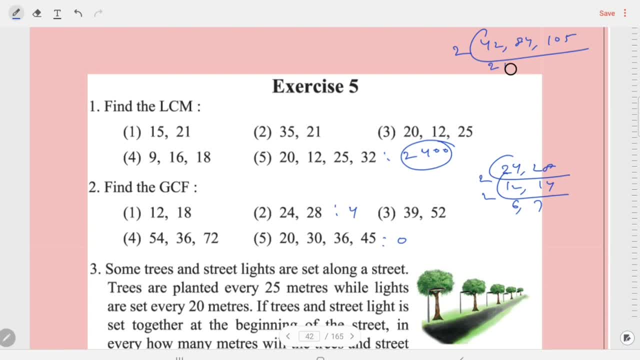 two. oh, okay, okay, three, three, one, two, three, three, four, two, three, four, two, twelve. three, two, six, three, eight, twenty four, three, three, three, three. three is a nine, three, five is a fifteen, seven, seven, two is a fourteen, seven, four is a twenty eight, seven, five is a thirty five. so